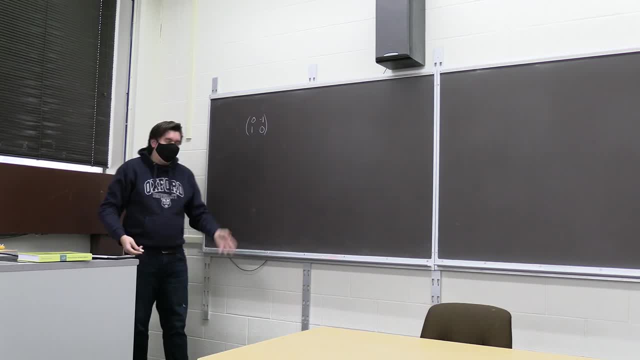 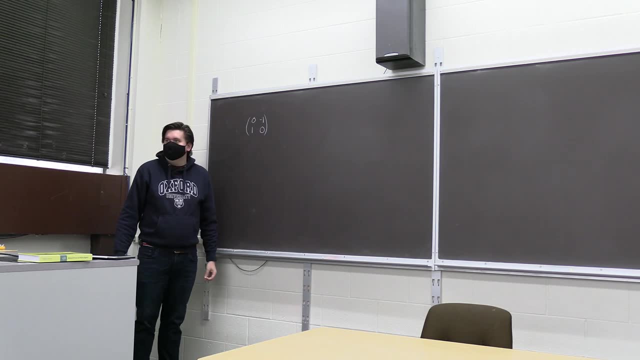 What other things do you do with matrices? You can find its transpose. That's great. What else? You can combine matrices. you can multiply them. you can look at its trace. Its trace is 0, the sum of its diagonal. 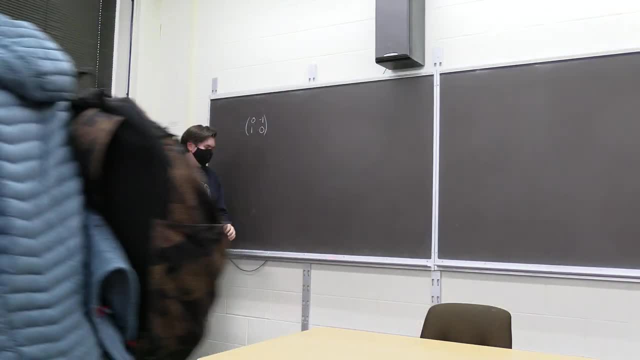 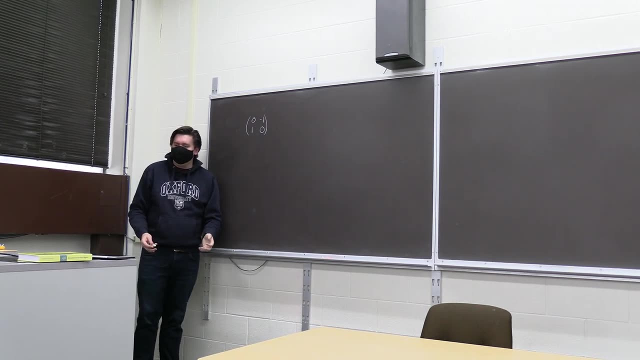 You can do all kinds of wonderful things with matrices. You can also come into class late, Okay, great. So you have like this study of matrices. but it's like: But if it's really just the studies of matrices, then like, why is the course called linear algebra? Shouldn't it just be called? 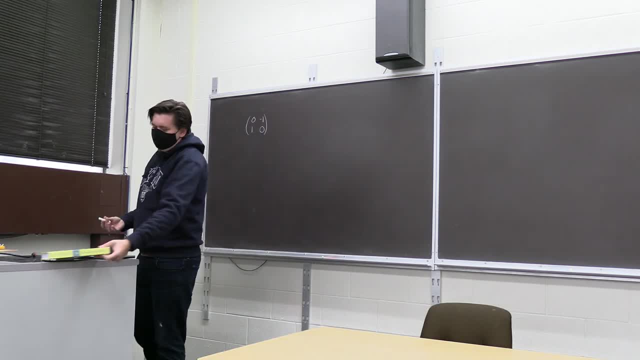 matrix algebra. And I mean, well, I guess a book for this course we're following quite closely is called Advanced Linear and Matrix Algebra. But what's the whole linear part about? It's like: well, this matrix isn't just an object, This matrix is encoding a transformation, right, We think? 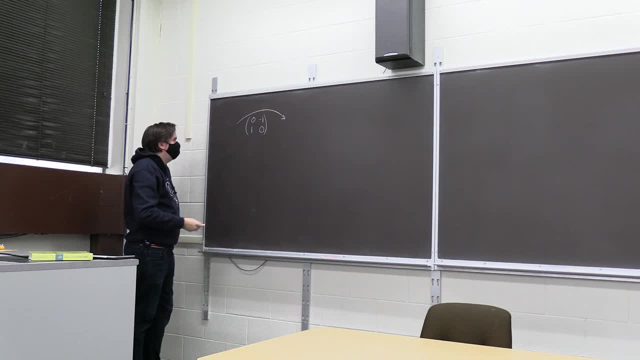 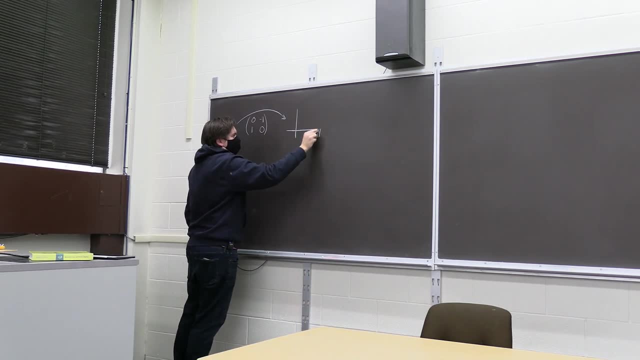 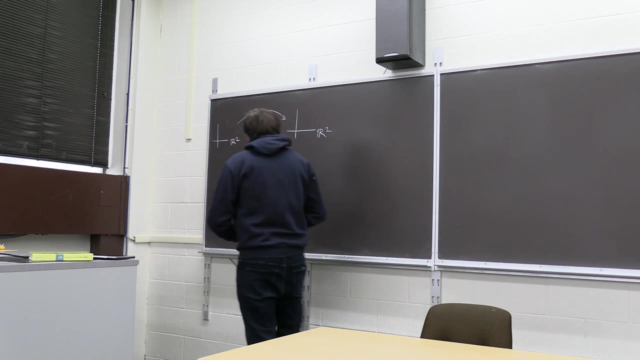 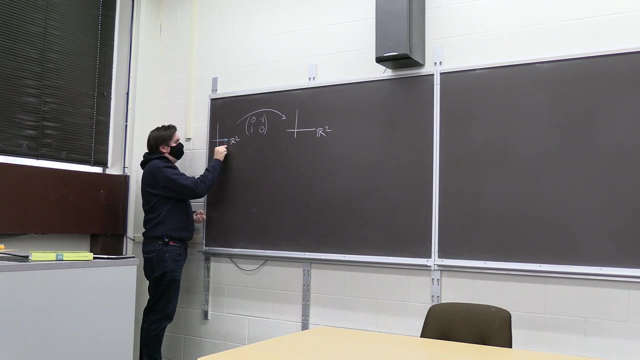 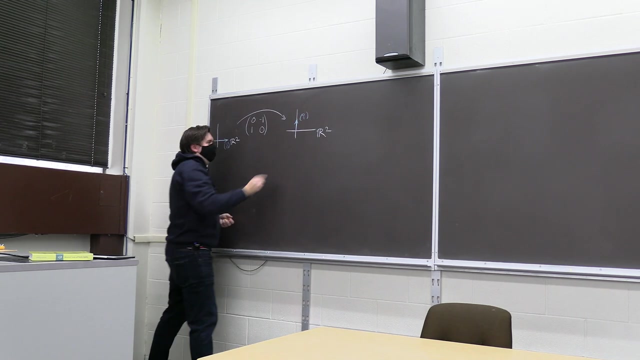 of this matrix as being a map between R2 and R2.. And the columns of the matrix are just telling you where your basis vectors, your elementary basis vectors. so here's some vector 1, 0. And this is telling us: 1, 0 gets sent to 0, 1.. And the vector, oh, I don't know. 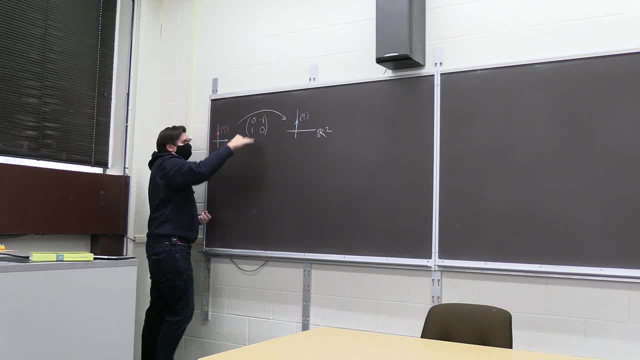 what is this guy? 0, 1 will get sent to negative 1, 0.. Negative 1, 0. And so it's like: what linear transformation is this? Which linear transformation is this? It's just rotating it. This is the transformation that's just rotating this guy by 90 degrees, or? 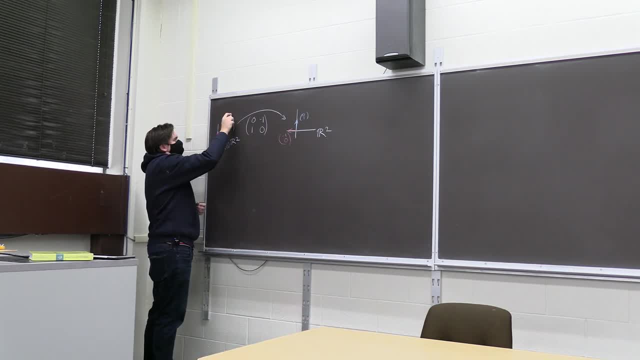 pi over 2 counterclockwise, right. So this is a 90-degree rotation. Okay, so the matrix is encoding some kind of transformation. I've been saying it's a linear transformation. What do I mean by linear? Well, what I mean is the transformation plays nice with various ways. 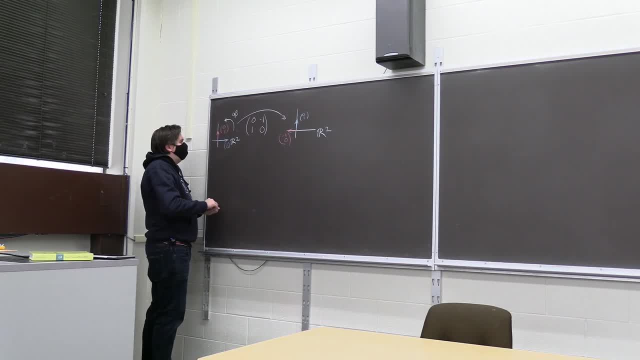 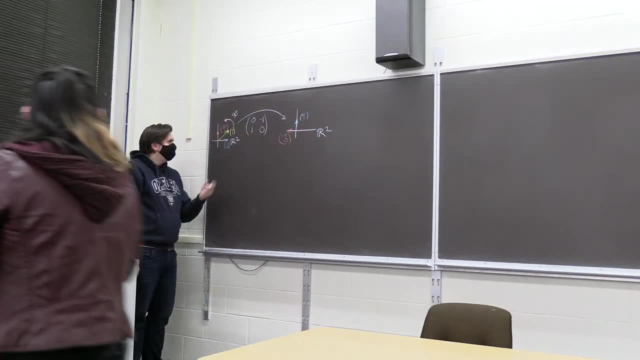 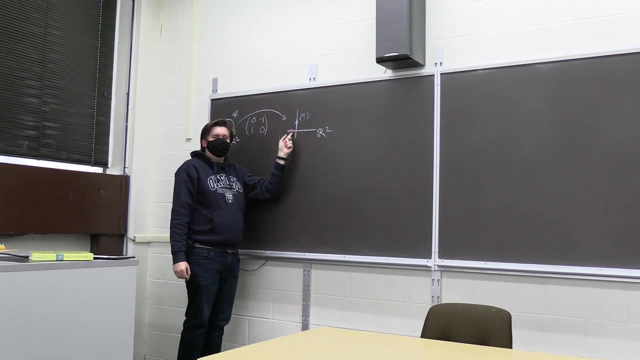 that you might try and combine these vectors. For example, I might look at the sum of these vectors to get the vector 1, 1.. And what does the rotation do to the sum of these vectors? Well, it gives me the sum of the resulting vectors. It'll give me the sum of the resulting 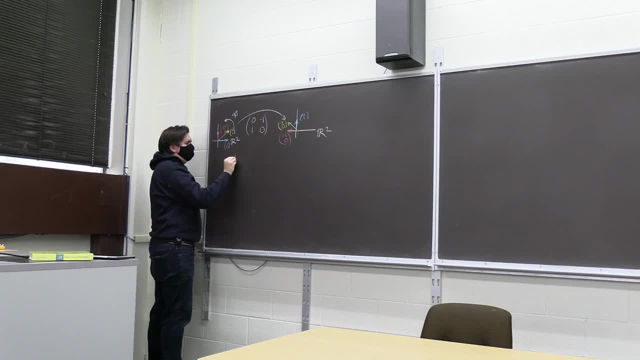 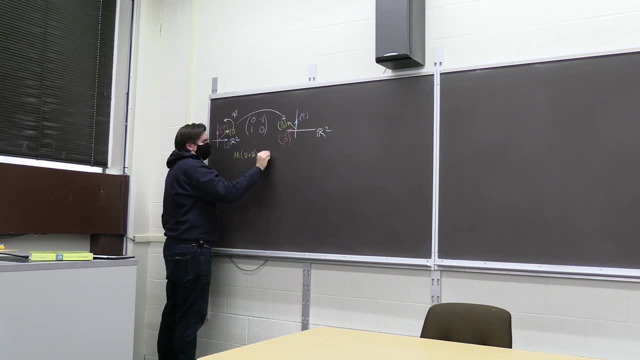 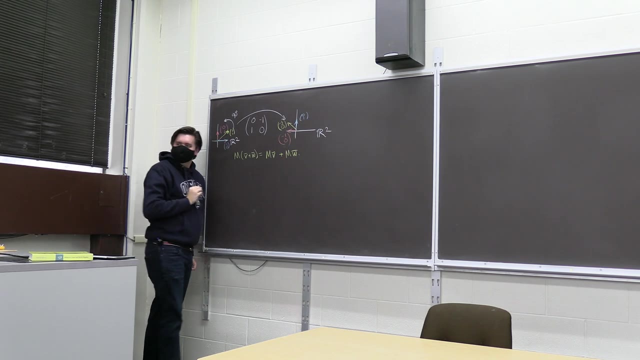 vectors. That is, when you have some matrix M applied to some vector V plus some vector W, what you get out is whatever the matrix M applied to V is plus, whatever the matrix M applied to W is Right. This is a really foundational property, And if we didn't have this, 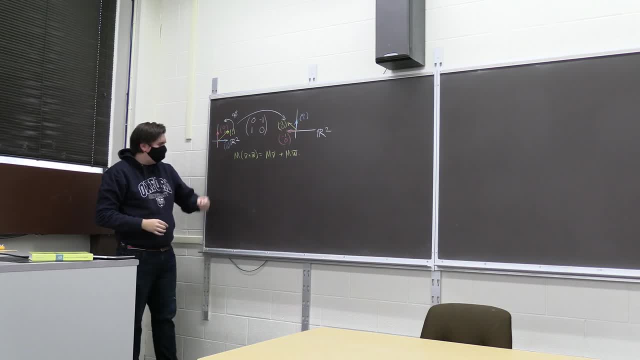 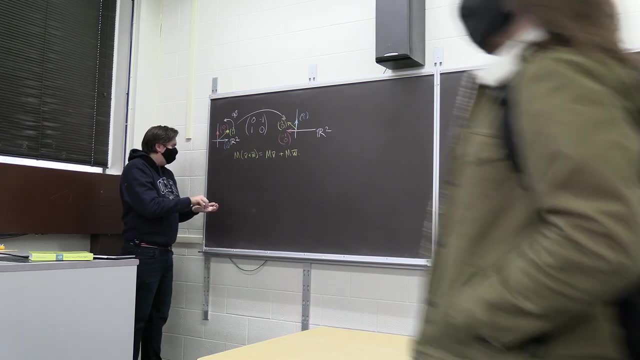 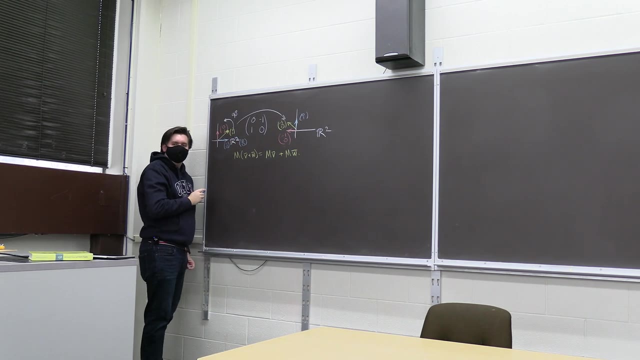 none of the things we said about these transformations would be true. So this is a really important property. And then we have a second property, If you want to imagine. oh, what if we doubled the length of this vector to be like 2, 0?? Yep. 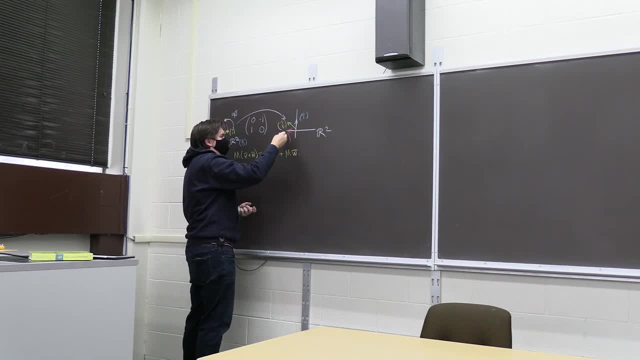 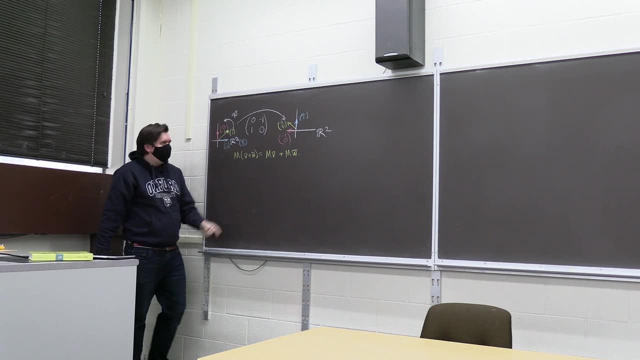 Yeah, this is negative: 1, 1.. That's right. It's the sum of these two vectors. Yeah, that's right. So what if I scale this vector by multiplying by 2? What would its image look like? Well, 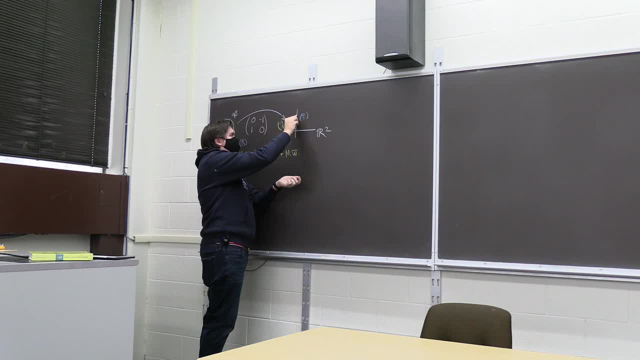 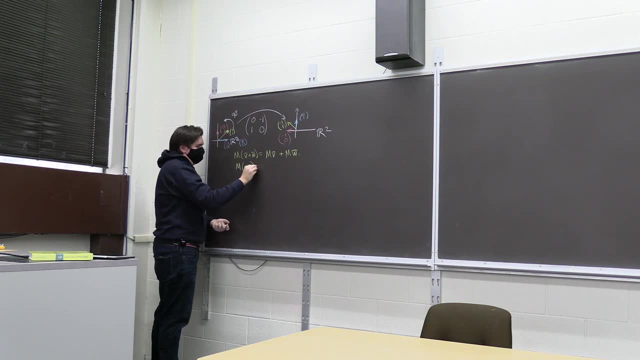 it's the same image but scaled by 2. So in some sense matrices respect scaling. That is, the matrix of some scalar copy of V is just that scalar copy of the image of V, Right? So these are like two really foundational properties of matrices. It allows you to say: if you have 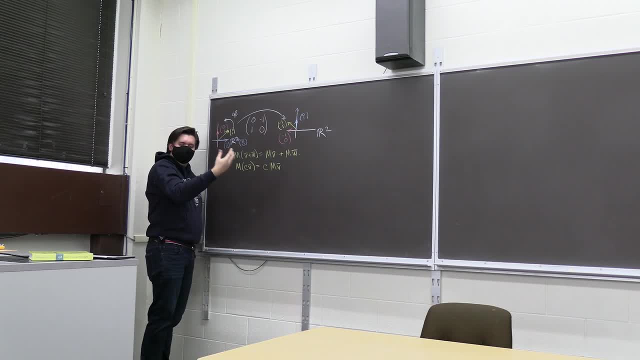 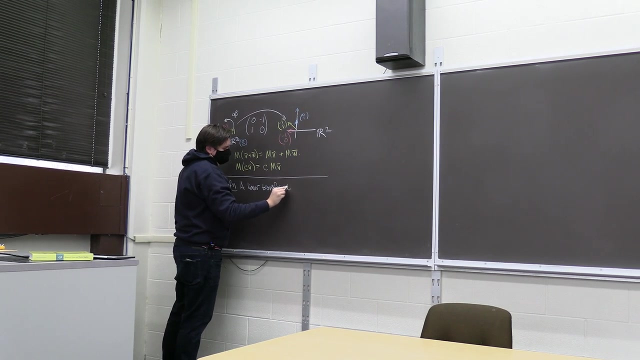 some linear combinations of things and you apply a matrix. it's the same as applying the matrix to each piece of the linear combination. So this is saying matrices play well with linear combinations. so we call a matrix a linear transformation, transformation More generally, definition, a linear transformation is going to be anything. 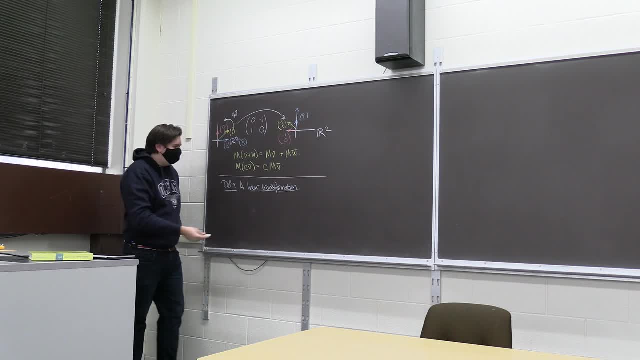 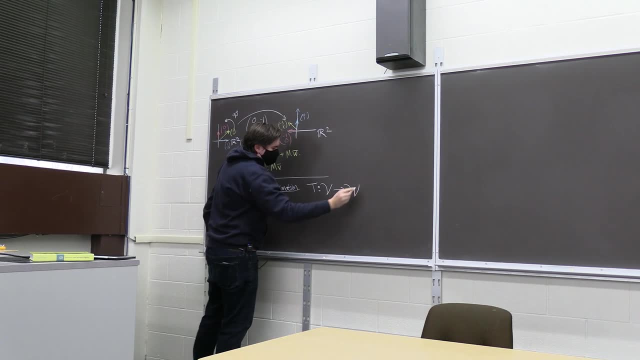 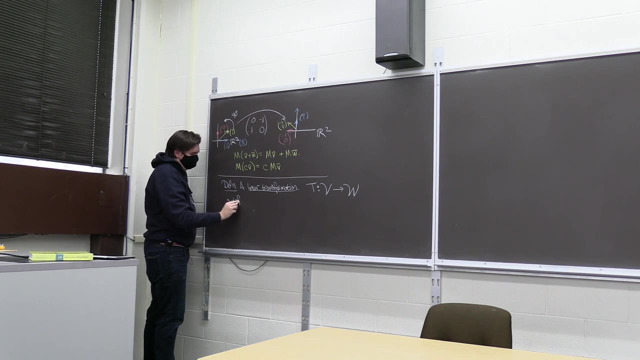 that has the same properties that matrices have: A linear transformation, some T from some vector space V to some vector space W. is some map from V to W that satisfies these two properties, The first property being the linear transformation applied to. well, we use the 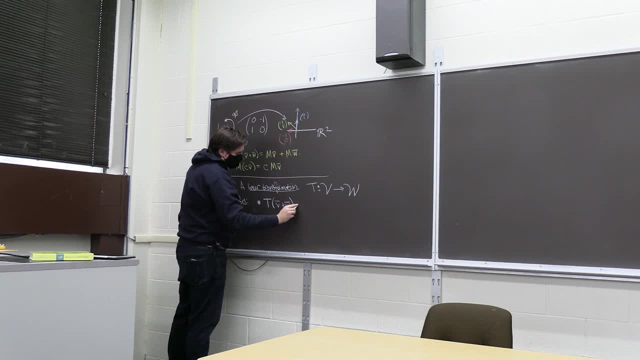 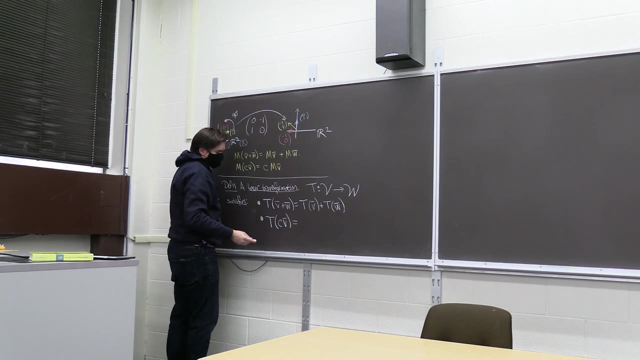 same language. V plus W is the linear transformation applied to V plus the linear transformation applied to W And the linear transformation applied to C times. V is C times the linear transformation applied to V, where our V and W are both vectors in a vector space, V. 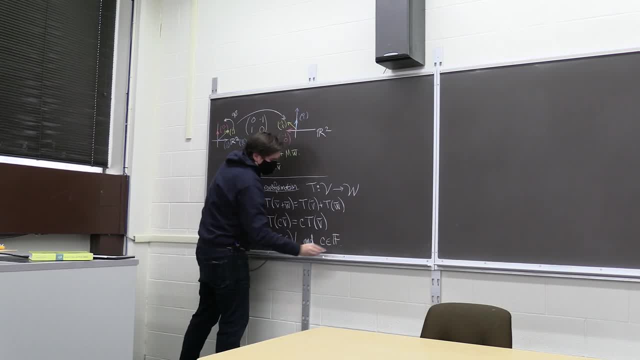 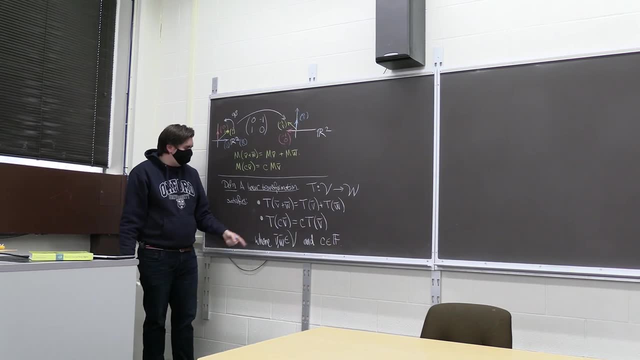 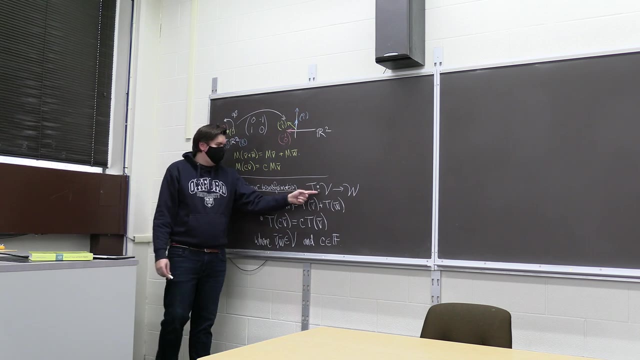 and our C is a scalar in our ground field. Now it is important that both vector spaces have the same ground field so we can make sense of what we mean by scaling by C, either before or after the transformation. So I'm assuming these are both, for instance, 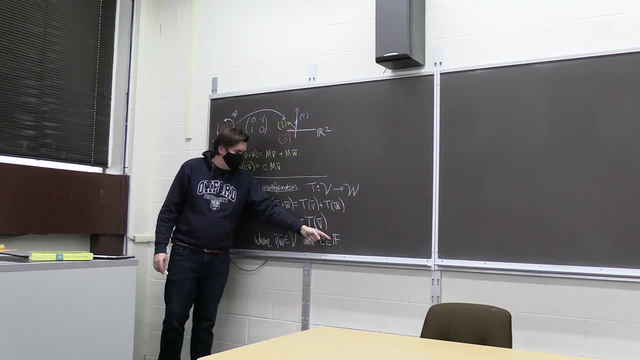 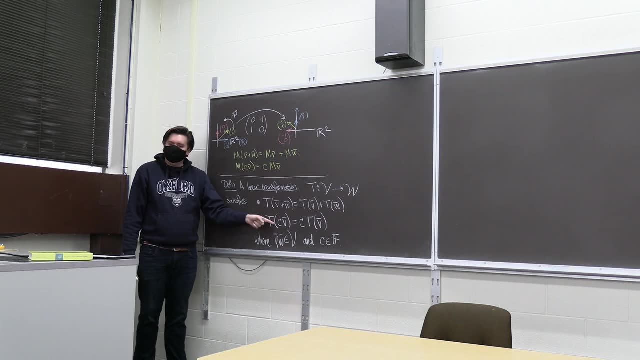 real vector spaces, vector spaces over the reals, or whatever the field of scalars is, should be the same. But given that I'm just going to say, linear transformation is anything that respects these two properties, which we might think are the essential two properties of matrices? 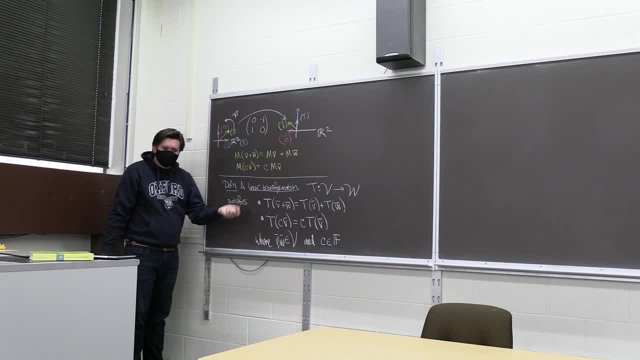 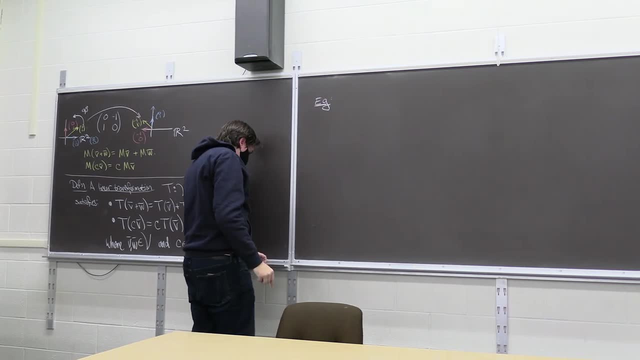 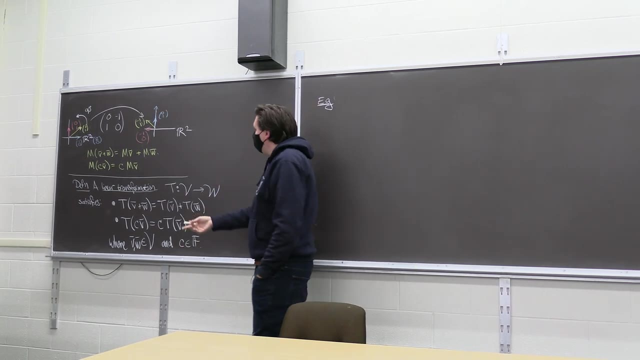 Okay. So let's look at some examples of this. So I mean, we've already seen the example of M, So let's maybe make that one a little more precise. Let's say M is a I don't know belongs to the class of 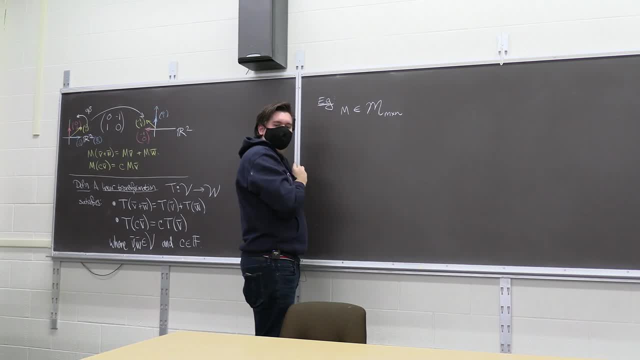 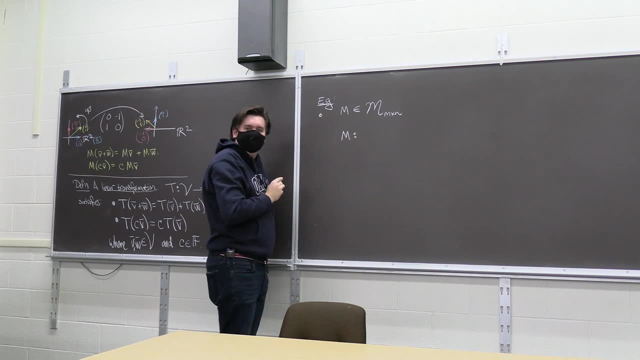 of M by N matrices. then we can think about M as being a map from where to where. Let's say, this is over the reals. From where to where It's a. yeah well, we gotta make sure we get the order. 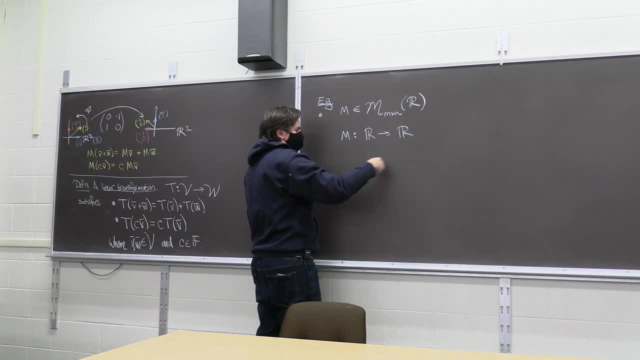 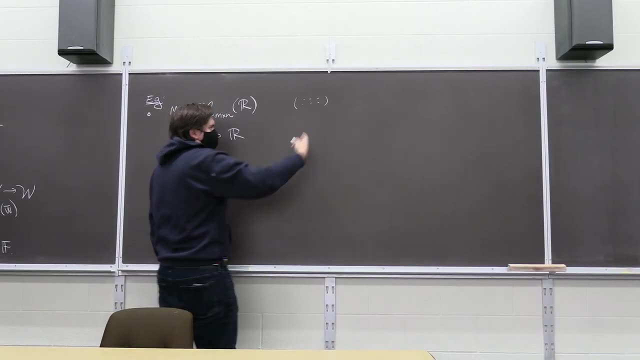 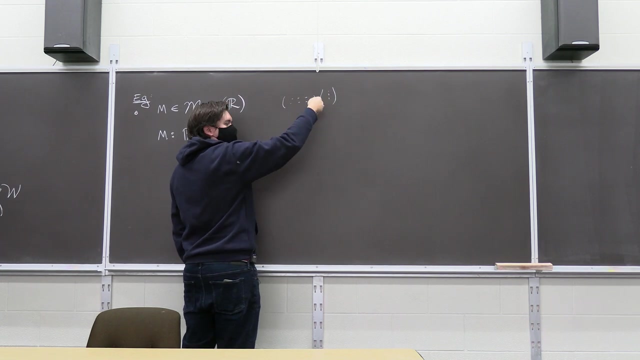 right between that M and that N, But here M represents rows, so like a two by three matrix would be like this: So what kind of thing will it eat in? Well, it should eat something that has three values, so you can do row times column. 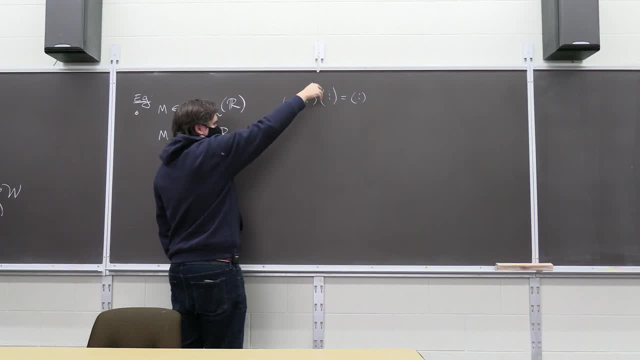 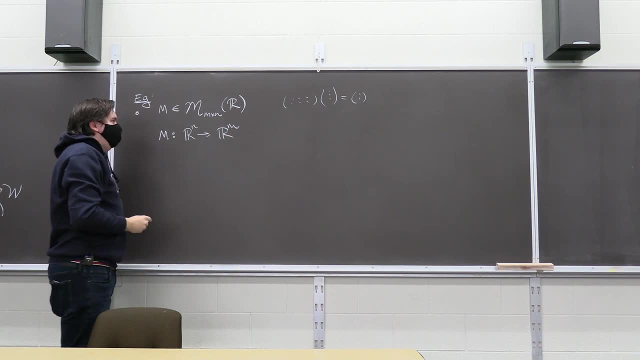 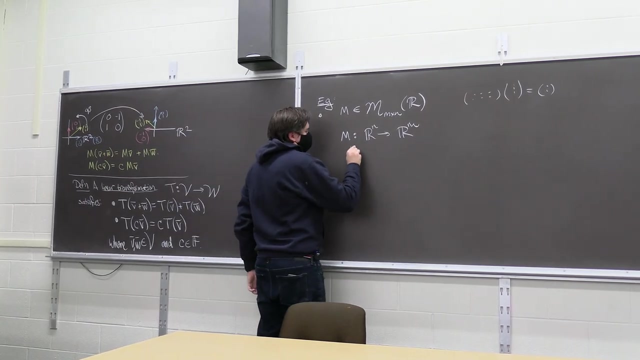 and then it'll spit out something with three rows and spit out some of two rows, right, so it's a map from our n to our m, and we've already seen that any matrix. you know, this was kind of a motivating example, but we've already seen that this is a linear transformation. this is a linear. 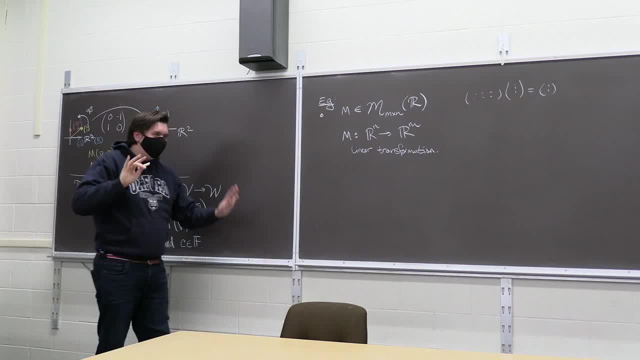 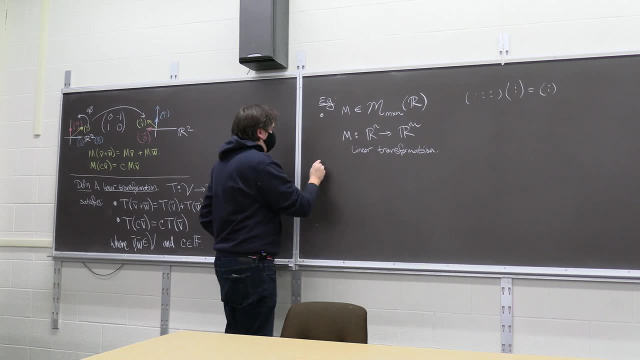 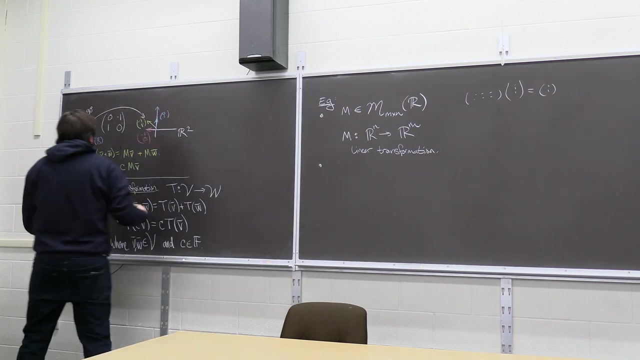 transformation. but don't think that, like, matrices are our only example of these guys. you might also just i don't know what is another transformation. well, at the beginning of class, i asked you guys like what are some things you can do to this matrix? and you named a number of. 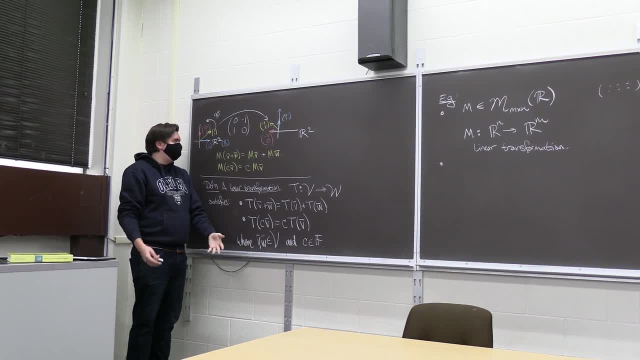 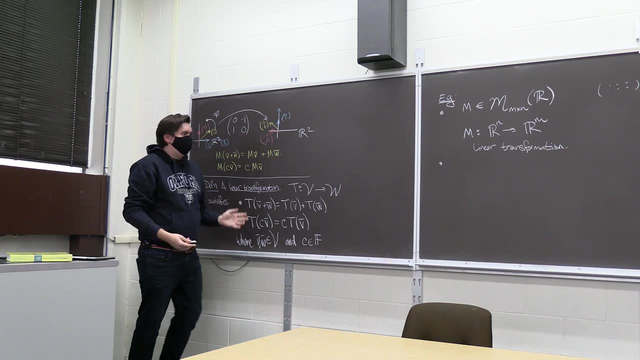 things you can do to matrices, and one of the things you said you can do is, for example, you can transpose them. you can. you can take the transpose of a matrix. so so what does it mean to take a transpose of a matrix? well, you can take a transpose of a matrix. you're changing an. 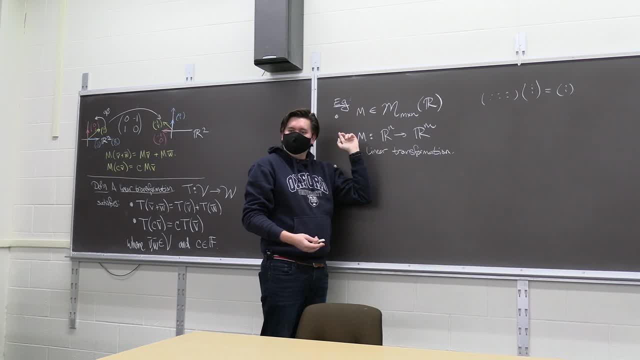 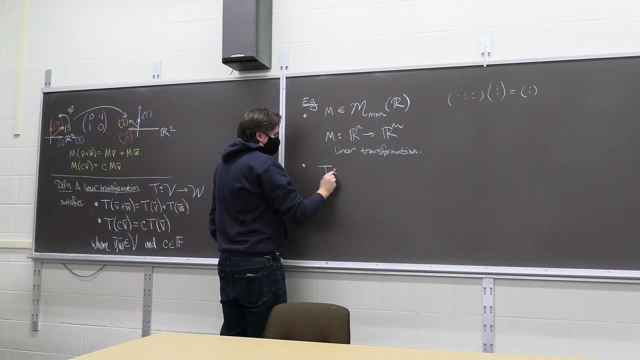 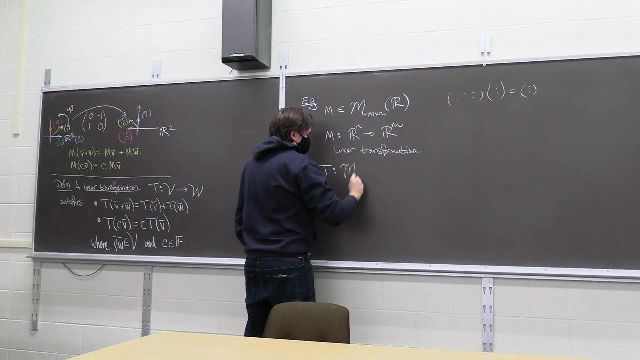 m by n matrix into a n by m matrix, right? so let's take a concrete example. let's think like t will be a transpose which, let's say, maps um, i don't know. let's restrict our attention to, like two by two matrices, so two by two matrices, to the collection of two by two matrices. 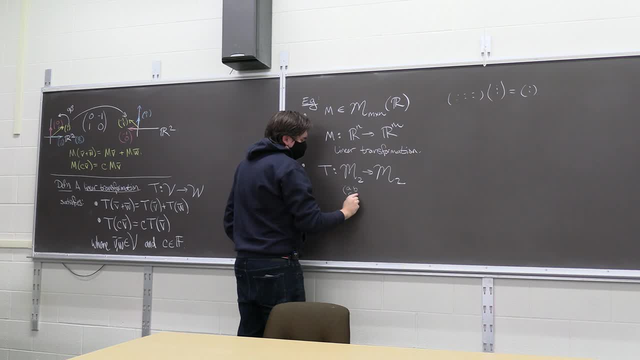 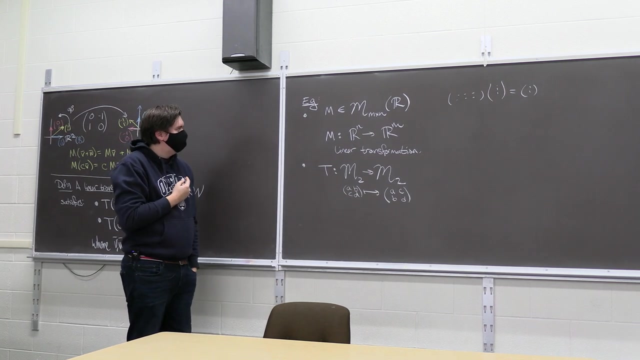 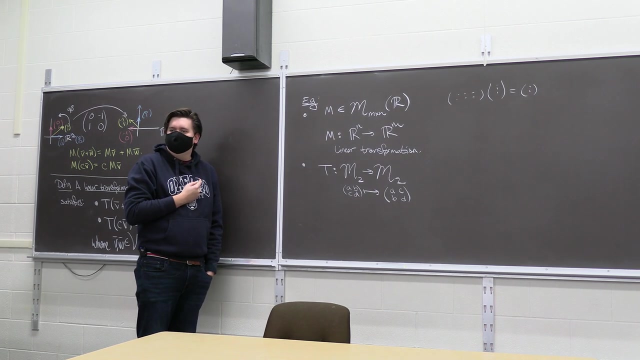 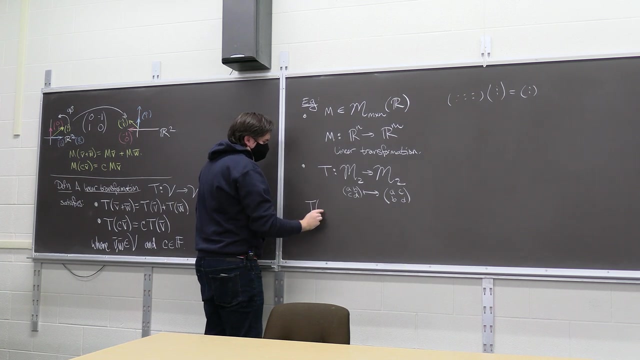 so. so this is the map that takes some a, b, d and sends it to some changing rows into columns, now column a, b, column c, d. this is the transpose map. is that a linear transformation? well, let's, let's take the transpose map of some matrix, i don't know, m. 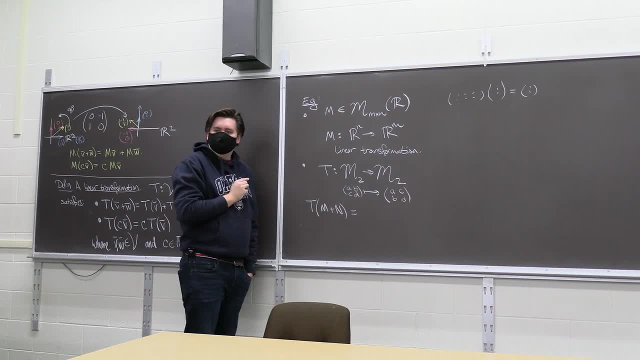 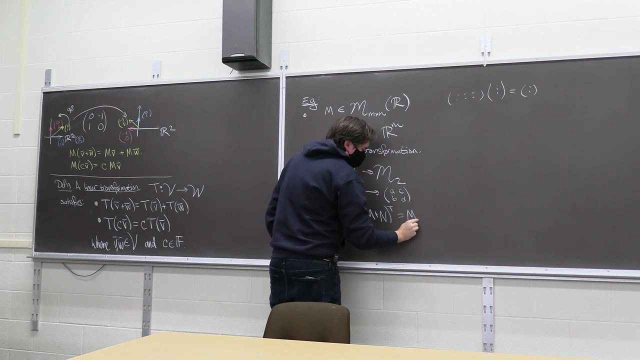 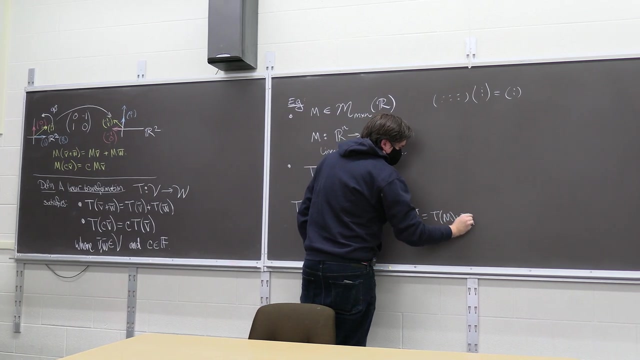 plus some other matrix n. what would that be? that's just m plus, and it's typical how you write it: transpose, right, but what is that? yeah, that's just m transpose plus n transpose, or the transpose map applied to m plus the transpose map applied to n. 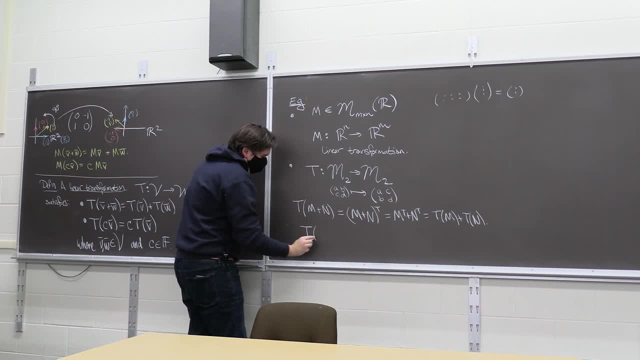 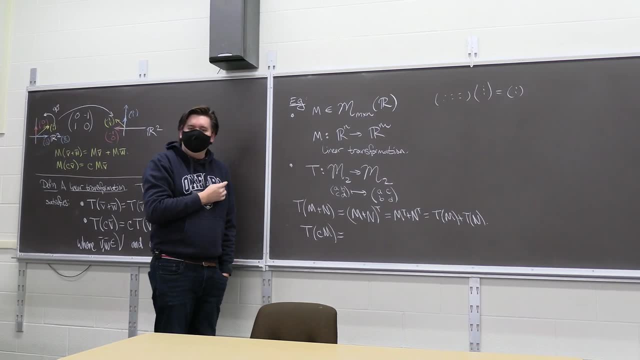 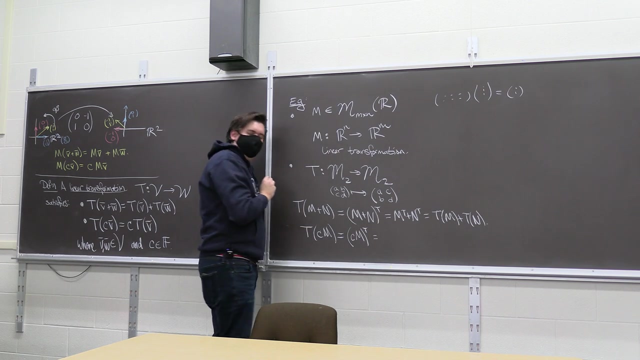 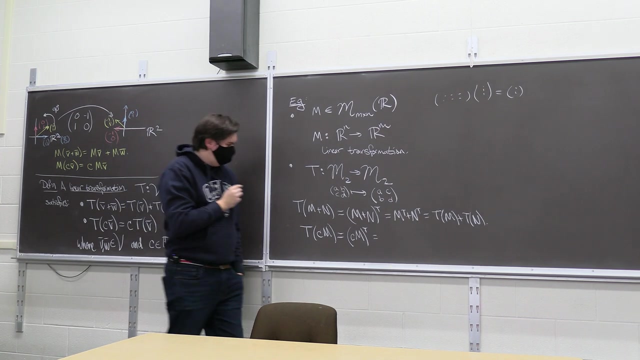 And what is the transpose map applied to some scalar copy of M, like 2 times M, for example? This is the transpose of some scalar copy of M. What would that be? Yeah, it's just a scalar copy of the transpose of M. 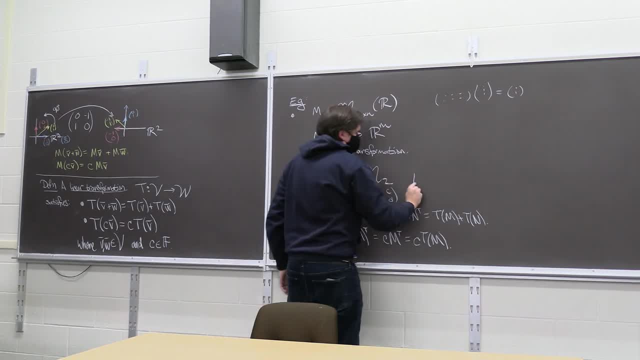 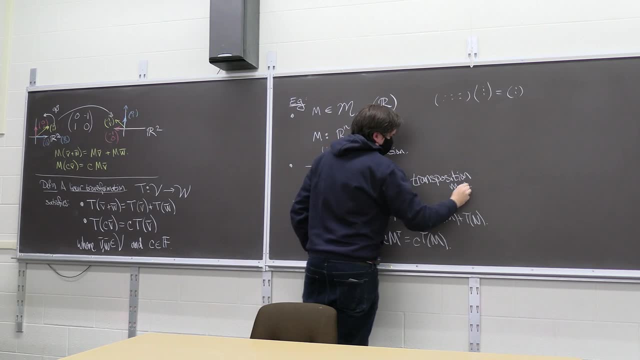 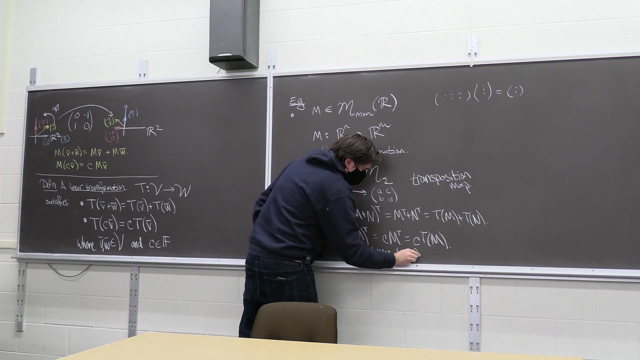 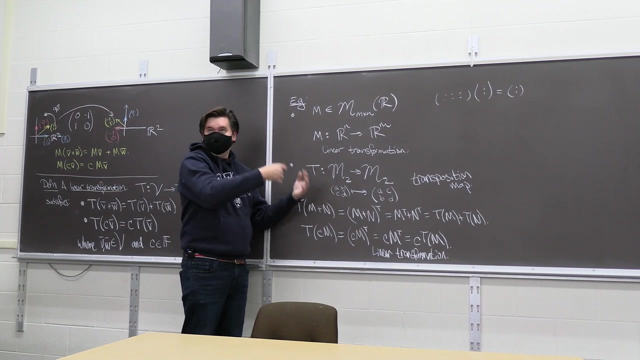 So this thing called transpose, the transposition map, is also a linear transformation. This is also a linear transformation From the vector space of whatever- 2 by 2 or more general N by N matrices, to M by N right. 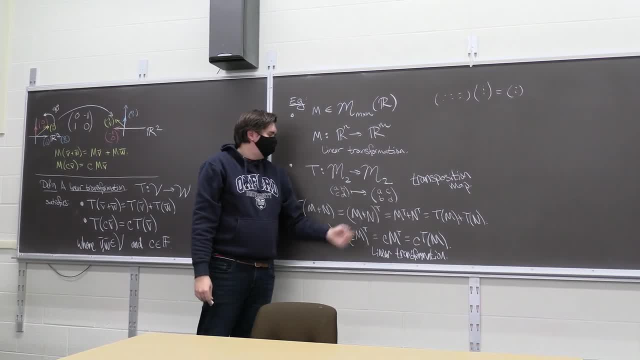 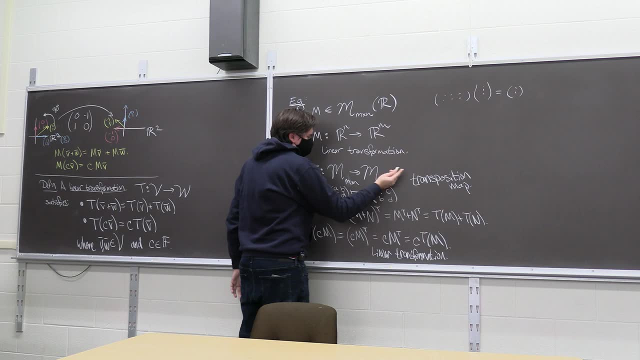 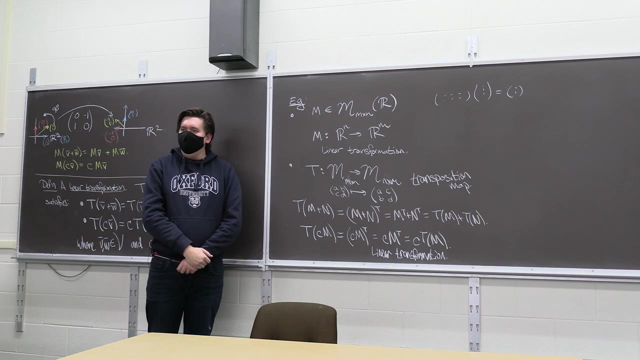 It just changes whatever the rows and columns are. So here's a 2 by 2 matrices, but you can generalize this from M by N matrices to N by M matrices if you like. Cool. So don't think it's like, don't think this is like our only kind of example. 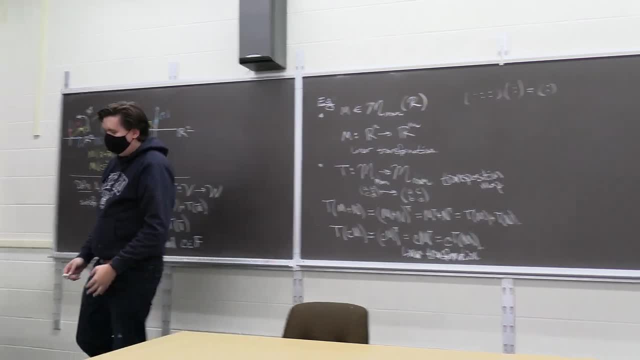 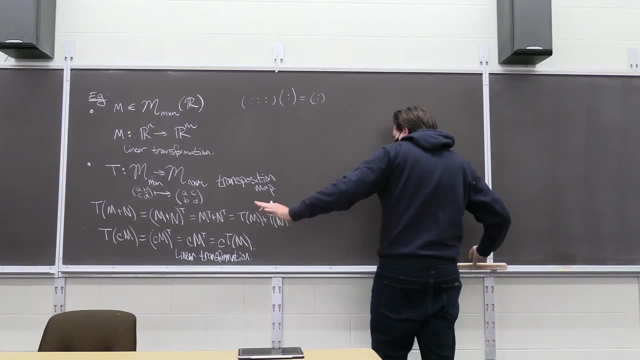 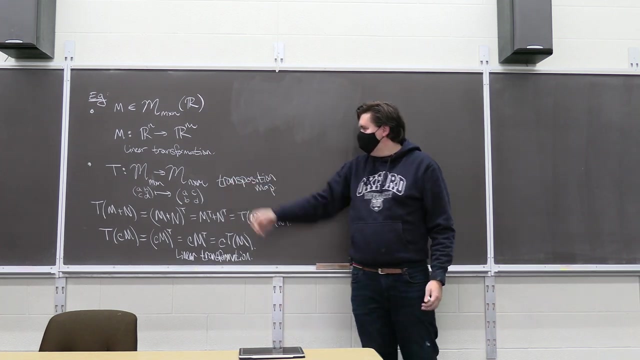 All other kinds of things are linear transformations also. Okay, can you think of any more? What is some other stuff that you do back in back in your first course in the algebra, other things you do to matrices. Let's check if those are also transposition maps or if they're also linear transformations. 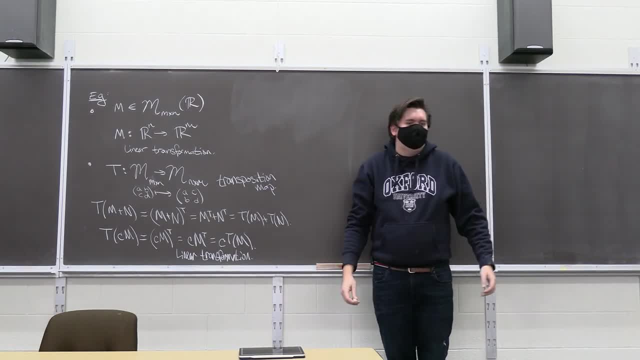 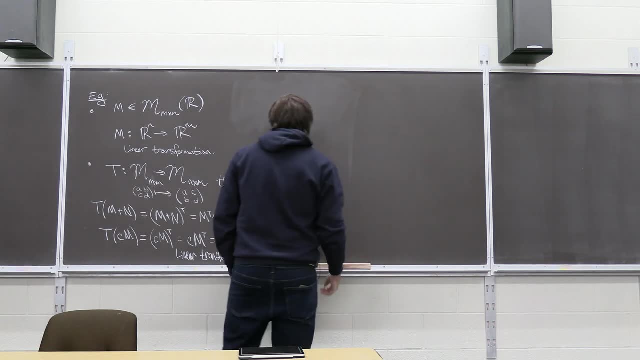 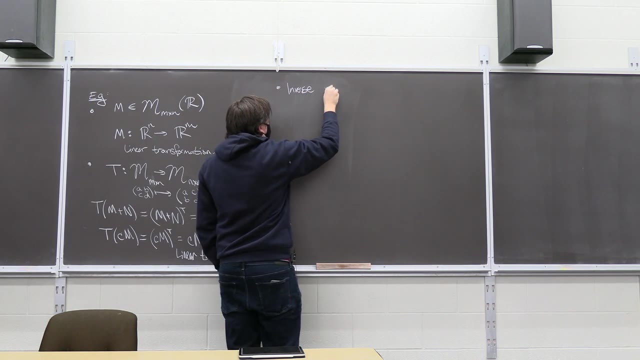 So, like, what's another thing you can ask about a matrix? Ah, you can ask if it has what the inverse of a matrix is. That's a cool question. So let's think about some kind of inverse map. So some kind of inverse map. 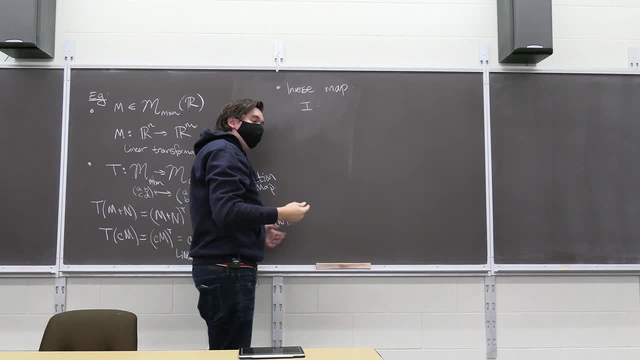 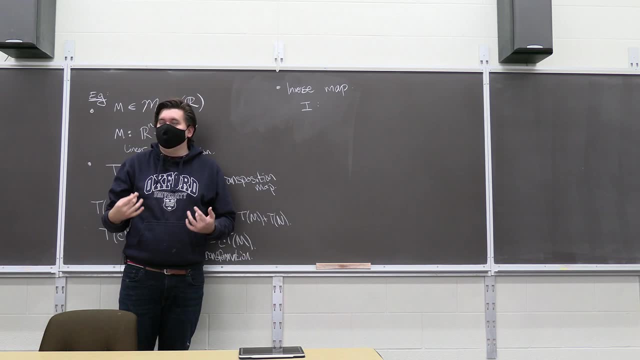 So I guess we could call this I And. well, it's only going to be defined on square matrices, right? And it would only be square matrices that have determinant non-zero. So I don't know, Have we introduced it, Have we introduced a notation for this? 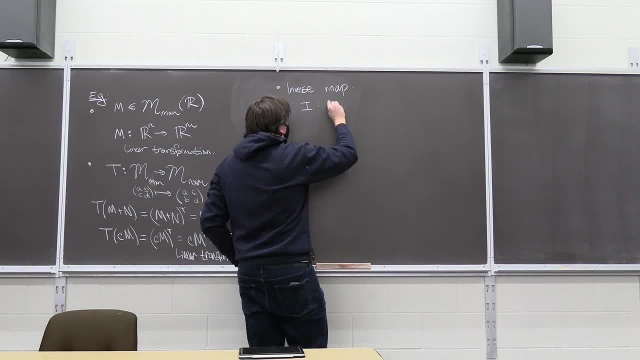 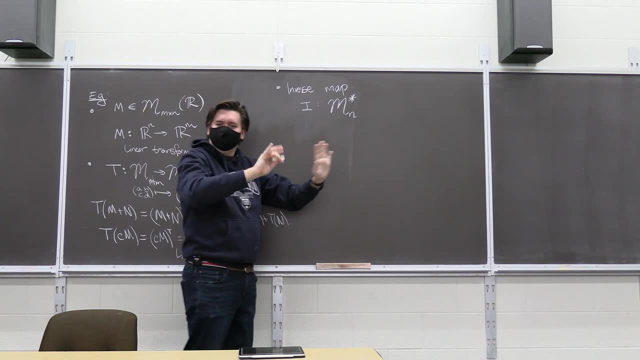 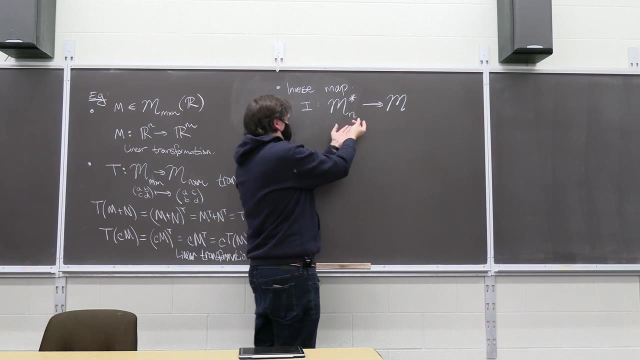 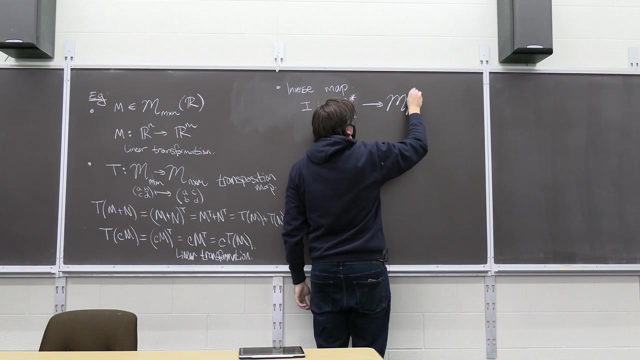 I don't know if we've introduced a notation for non-singular square matrices, So let me introduce a notation for this. I'll do a little star here. by mean non-singular square matrices, matrices with determinant non-zero, And we'll map those to. well, if you start with an n by n square matrix, that's non-singular, you take the inverse, you get out an n by n square matrix, that's non-singular. 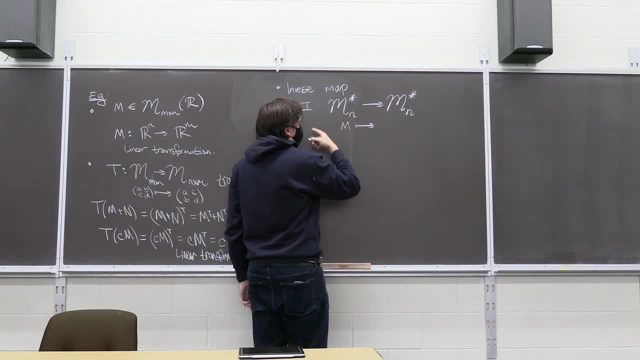 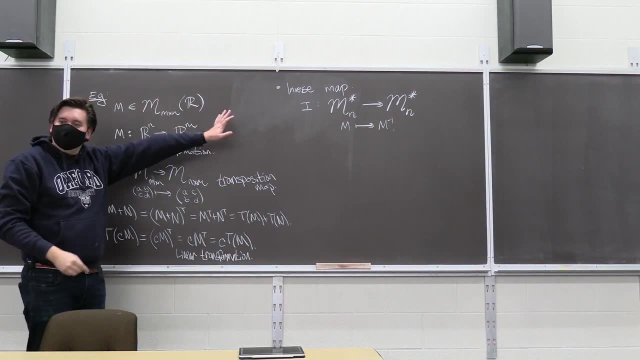 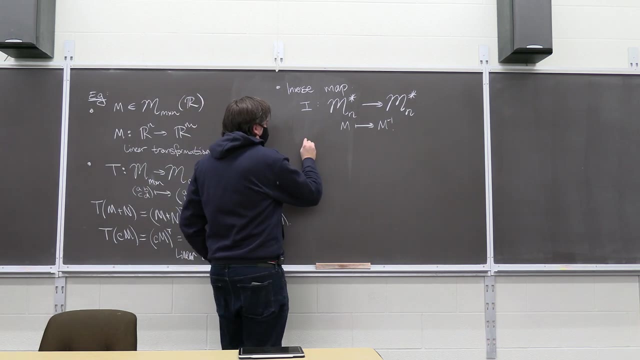 That is, you take the inverse, you get out an n by n square matrix. that's non-singular. You take in some matrix M. this map sends out M inverse. So is that a linear transformation? I mean, let's check. 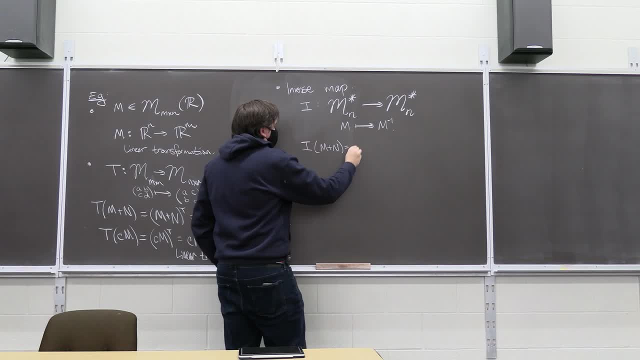 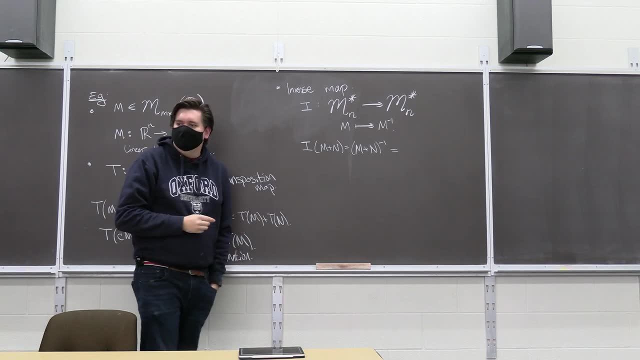 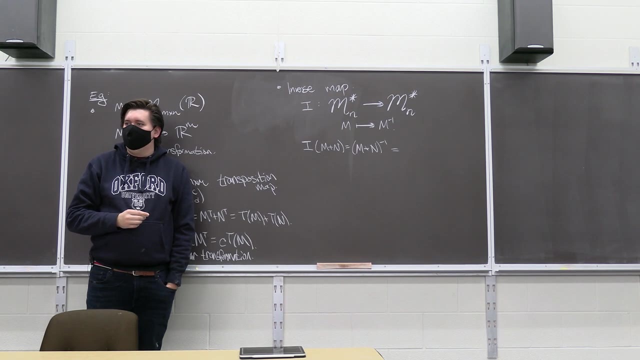 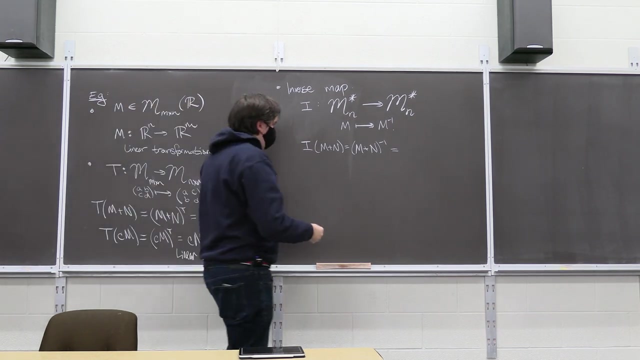 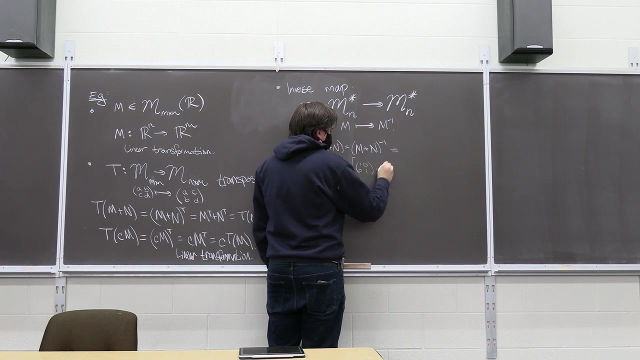 What is I to like? some matrix M plus some matrix N. Well, that's M plus N inverse. Is that M inverse plus N inverse? Yeah, No, Maybe we should just do a concrete example, Like: what's the inverse of your identity matrix plus your identity matrix? 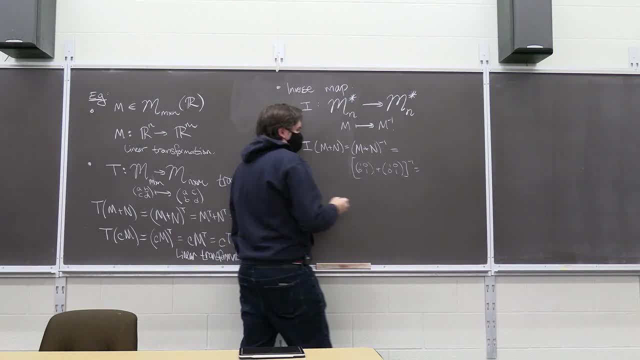 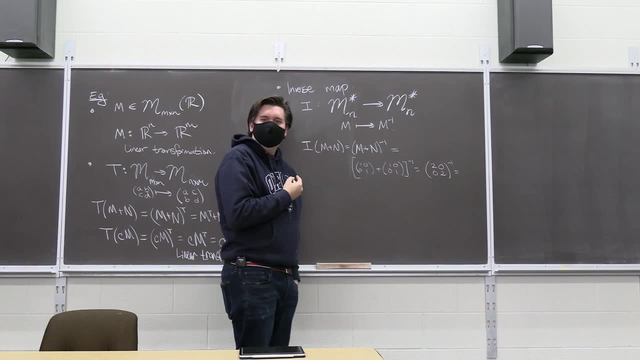 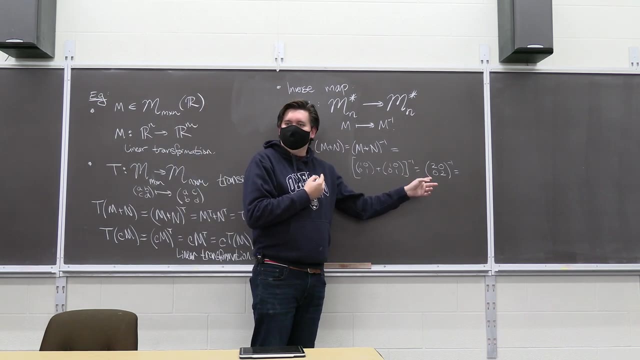 That's the inverse of your identity matrix. That's the inverse of your identity matrix. That's the inverse of the matrix 2, 0, 0, 2.. What's the inverse of that guy? Well, you need a one over determinant, right. 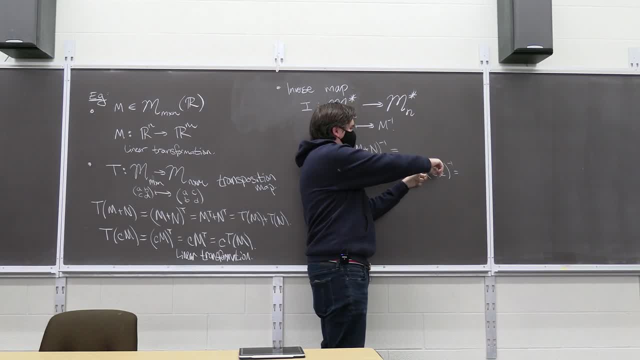 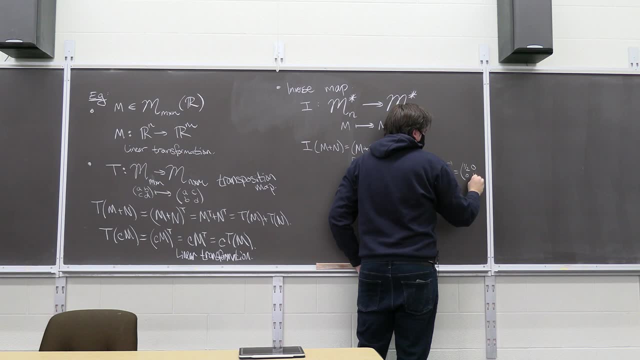 So we're going to be multiplying one-fourth times And then, when you do like the switching, it's going to stay the same. So it's one-fourth times this matrix. So, exactly right, it's just one-half 0, 0, one-half. 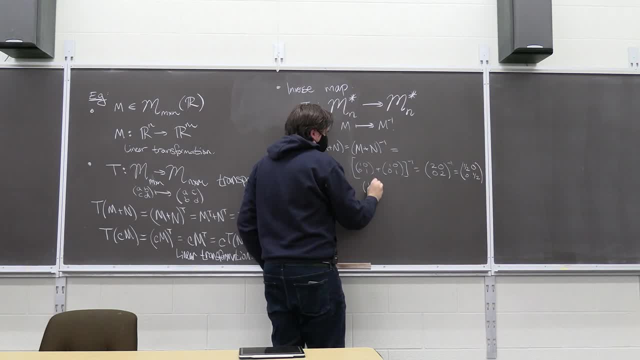 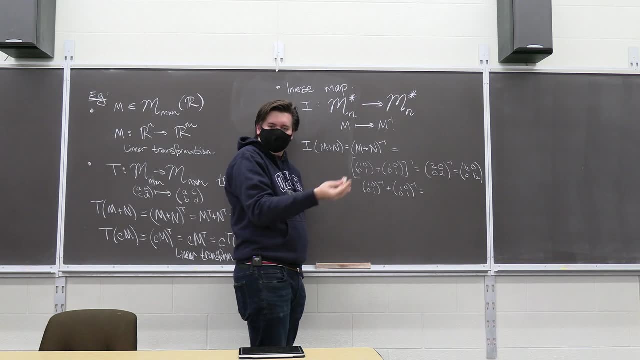 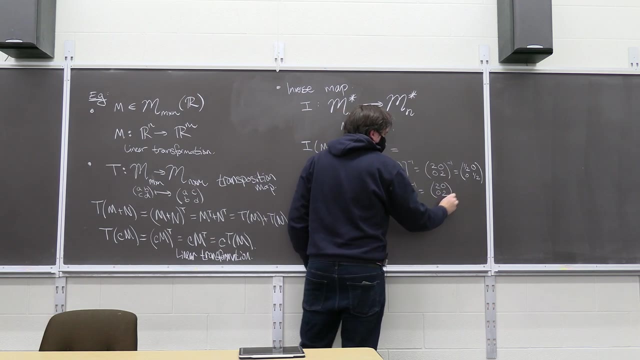 By way of contrast, what is inverse of identity added with the inverse of the identity matrix? Well, the inverse of the identity matrix is just the identity matrix. So this is the identity matrix plus itself. So this is 2, 0,, 0,, 2.. 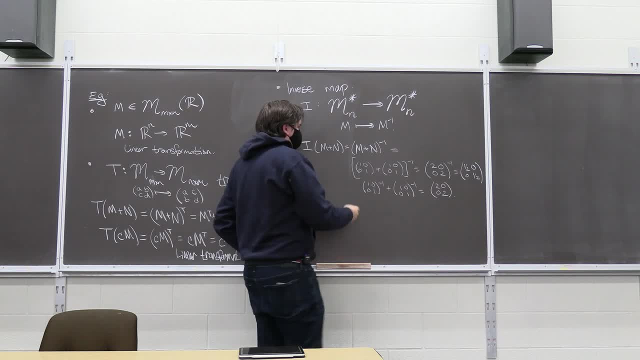 So it fails there and, more broadly, you can't expect it to work. So this is not, in general, equal to M inverse plus N inverse. Yeah, it's an interesting question. When is it equal? You can try and think about the set of matrices. when this is true, 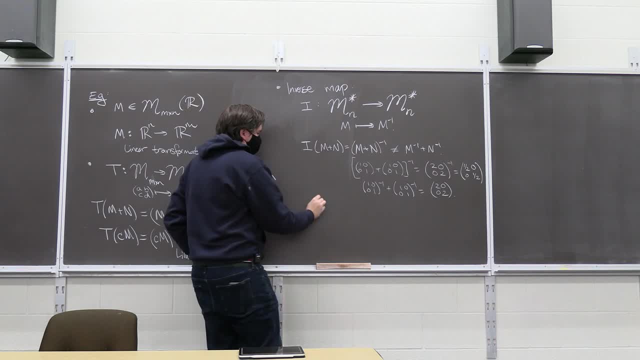 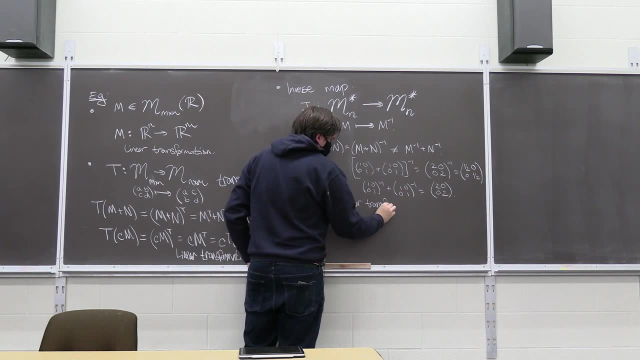 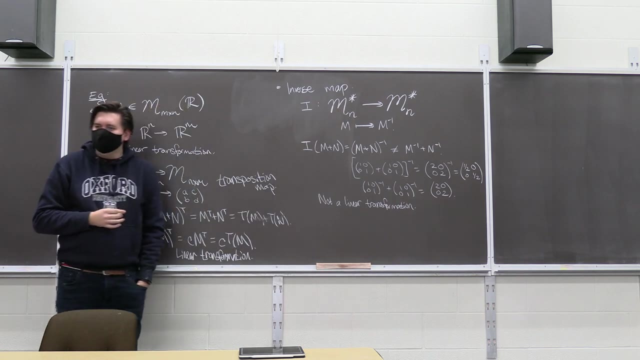 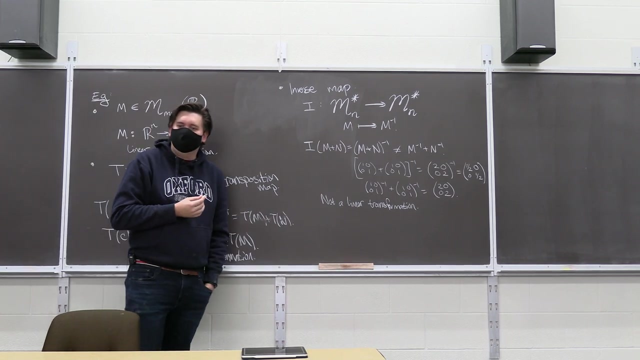 That could be a fun little thing to think about, But in general, this is not So. this is not a linear transformation. I'm just quickly thinking about one or two more. What other things do you do to matrices, Other things you can ask about a matrix? 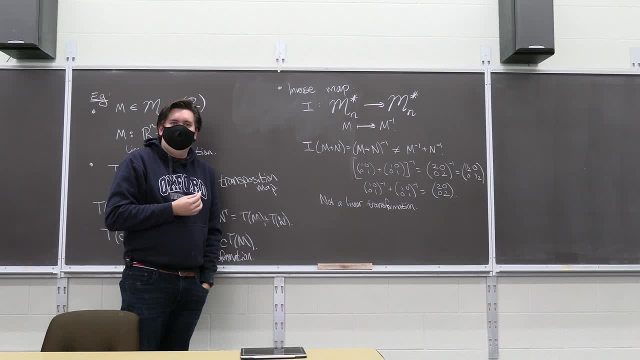 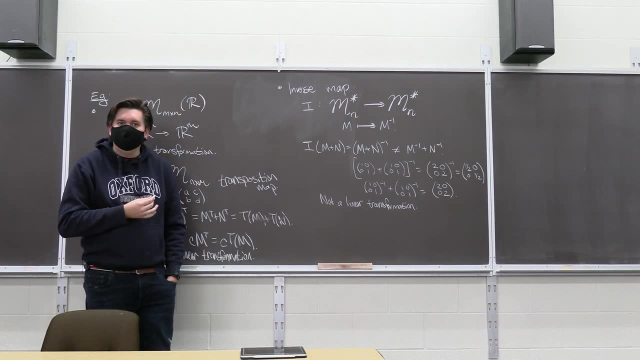 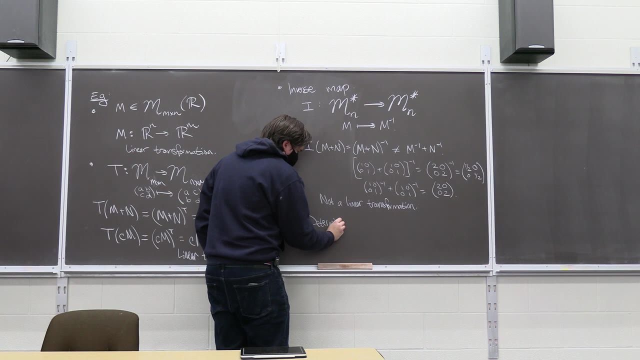 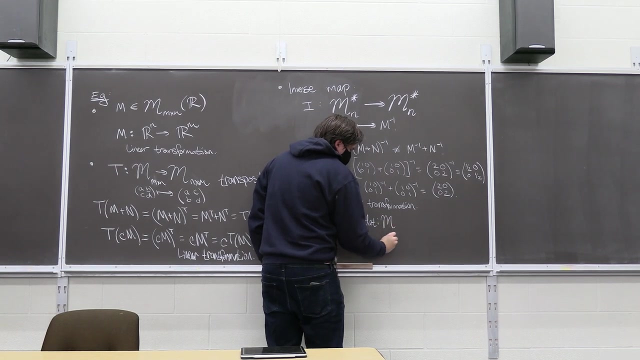 Determinant, Determinant, Will determinant be a linear transformation. So this determinant map- I'll just call it det from. well, again, we should have some square matrix, some N by N matrix, And what kind of things are going to spit out? 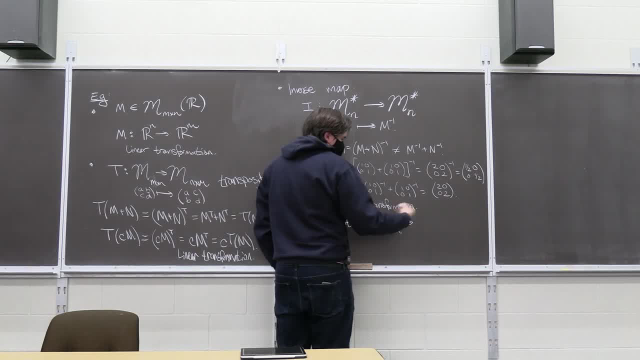 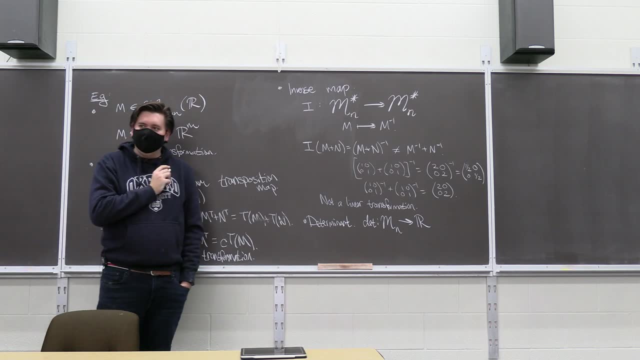 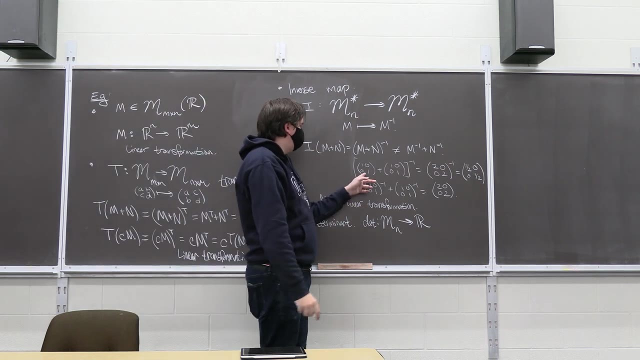 Well, if these are matrices of real value entries, it'll spit out a real number. So the map looks like this: Does that one work? No, And I mean you can even just go up to this one. The determinant of this guy is 1.. 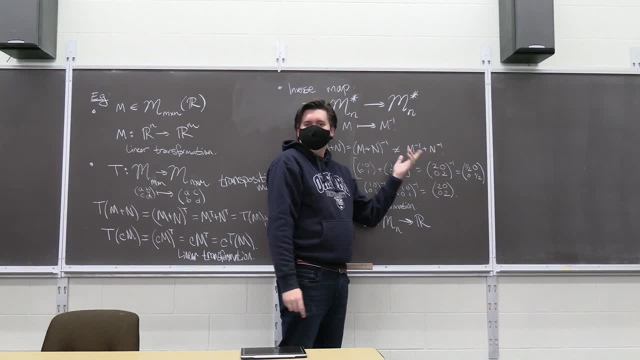 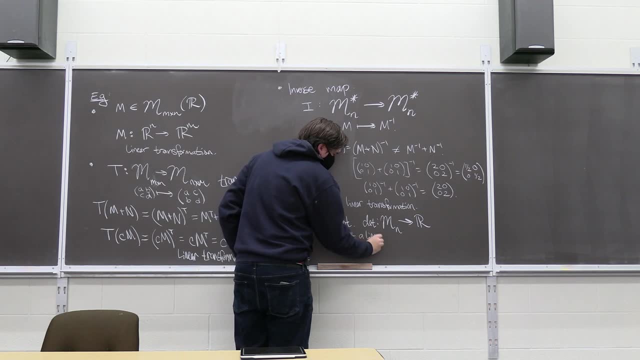 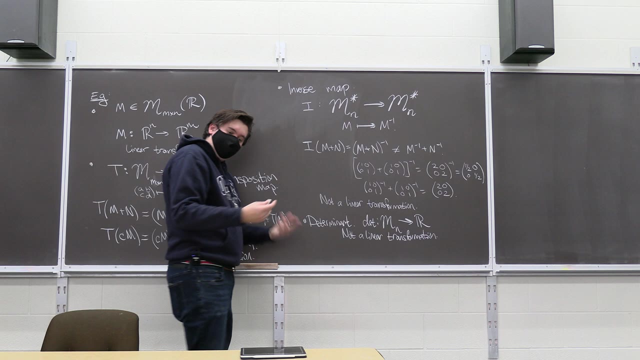 Determinant of this guy is 1.. But the determinant of their sum is 4.. So this is also not a linear transformation. Not a linear transformation, Linear transformation. It also doesn't work well with scaling. If you scale a matrix by 2, it means you're multiplying all the columns by 2.. 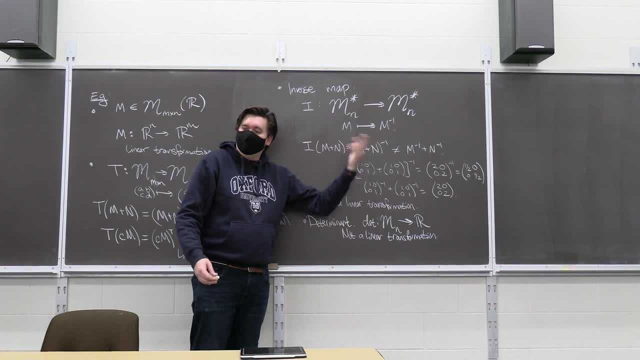 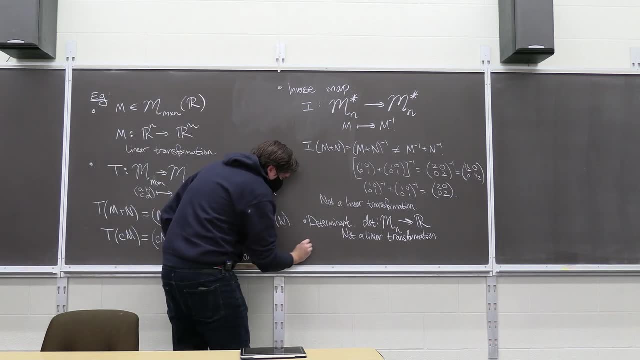 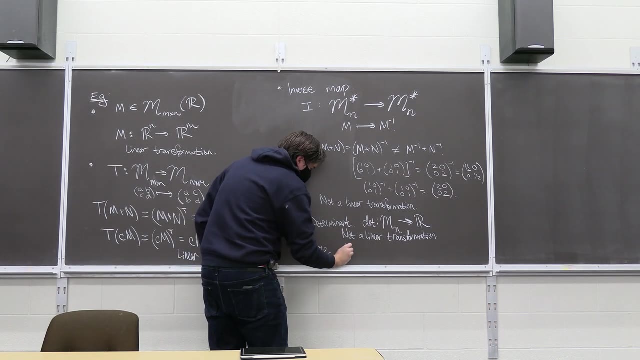 So the matrix actually gets the determinant gets multiplied by 2 to the N, One for each column. So determinant's going to fail. How about trace? So again the trace is going to look at. maybe let's call it the map TR. 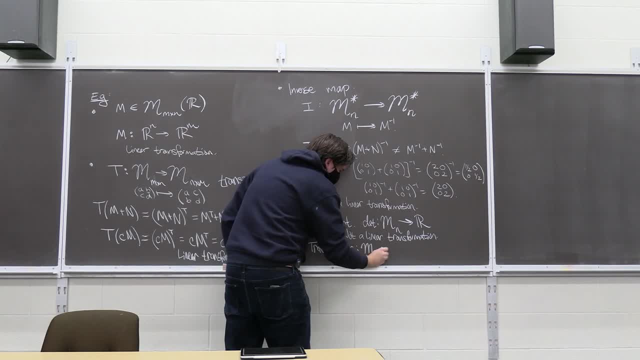 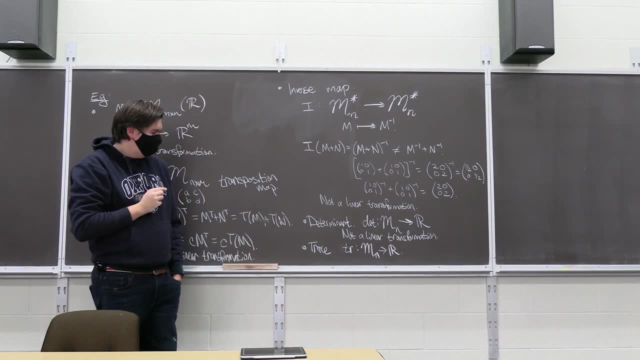 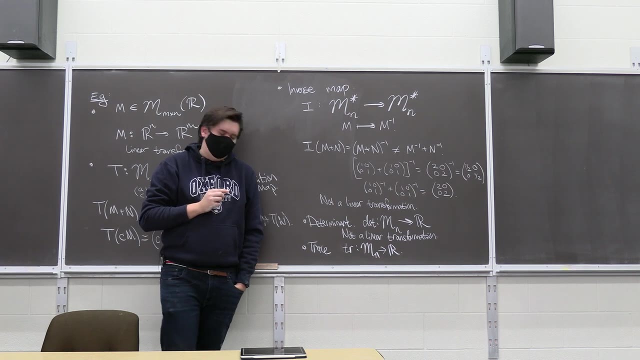 It's going to be the map of N by N matrices. say, to the real numbers You just add up the diagonal entries. Is that a linear transformation? Yeah, If you have the diagonal entries of one matrix, you add another matrix. 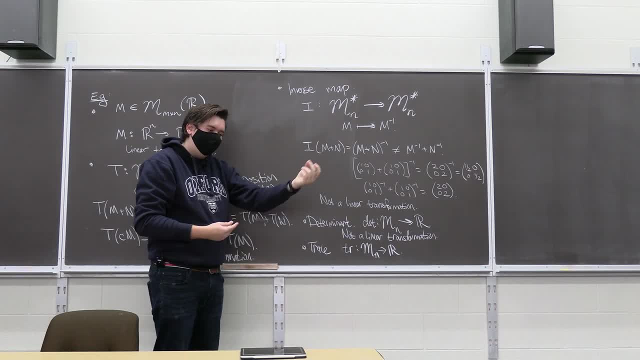 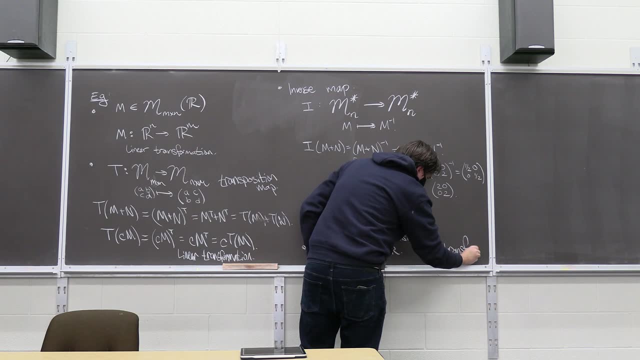 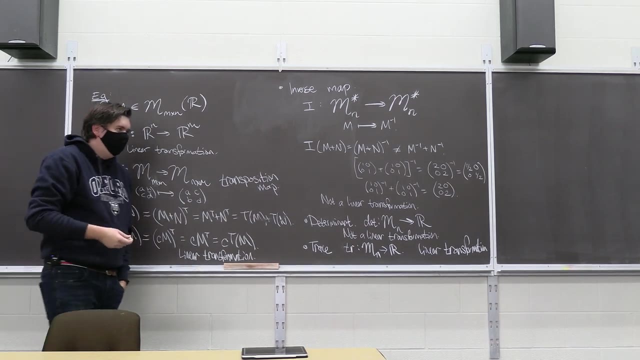 You're just going to add the diagonal entries. If you're scaling, you're scaling the diagonal entries by that thing. So this is a linear transformation. Okay, So we're seeing lots of examples and non-examples of linear transformations. Hopefully it's been an intuition. 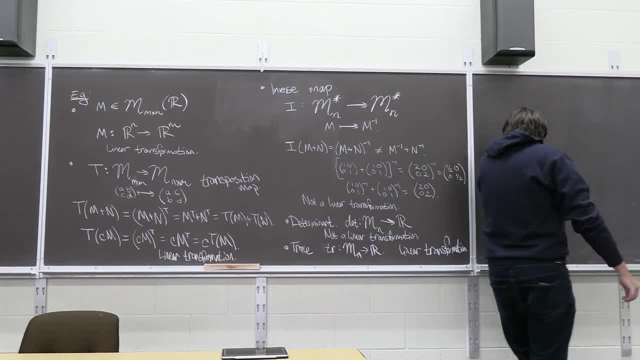 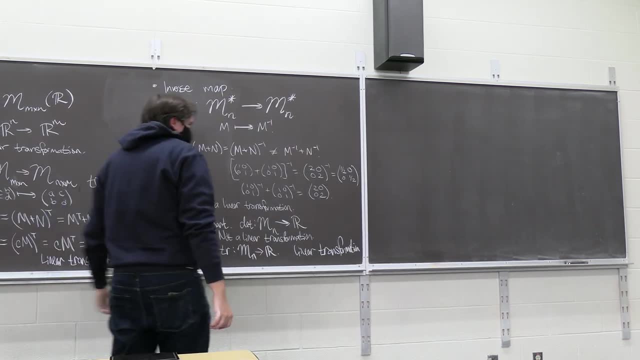 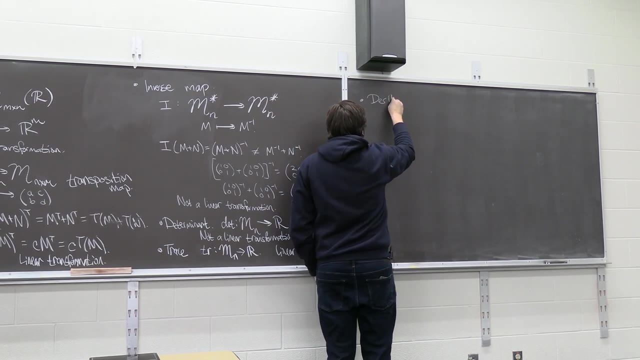 Let me just give you one more. Let's forget about linear algebra. I mean, there are other classes you've taken right Like you probably did a bit of calculus in your day. So what if we think about something like the derivative map? 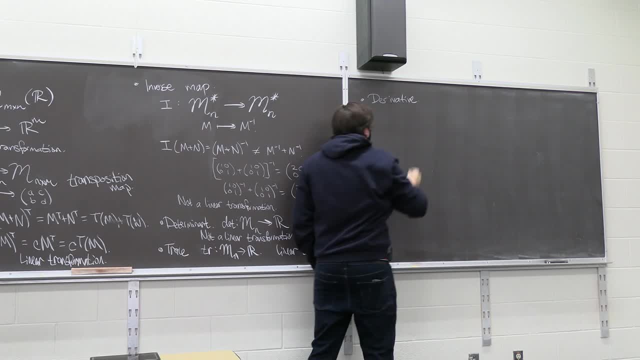 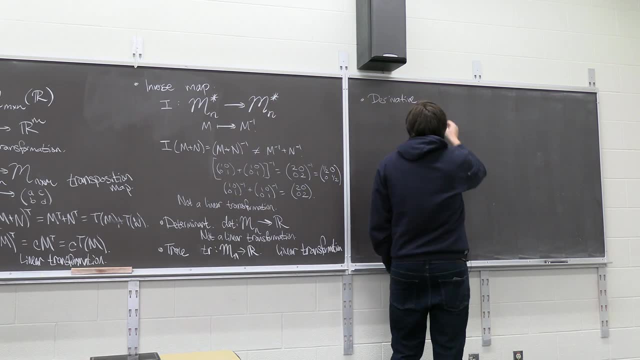 Derivative. Is the derivative a linear transformation? So you might think of the derivative as being some map from. I don't know. I should specify: this is like a map from. you can only take the derivative on functions that are differentiable. 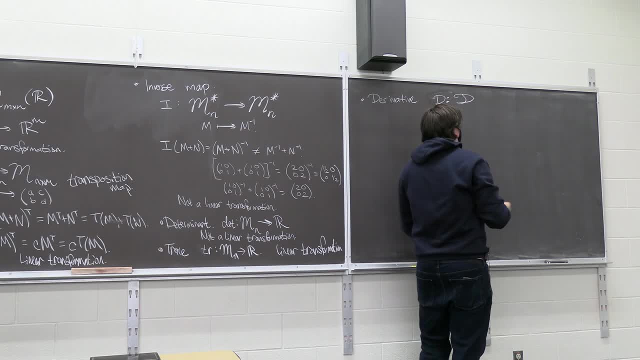 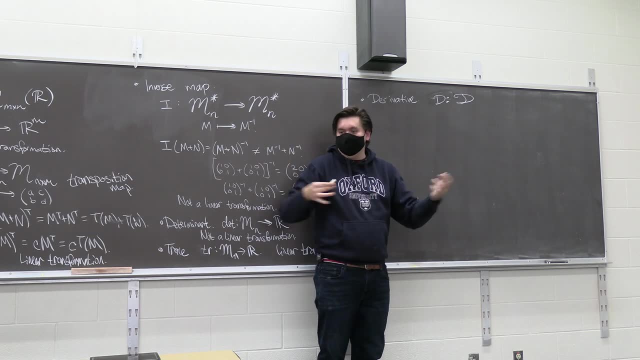 So let me introduce some notation, fancy D to introduce, like the vector space of differentiable. Well, is that really a vector space? If you add two differentiable functions, it's still differentiable. If you scale a differentiable function, it's still. yeah, that's a vector space. 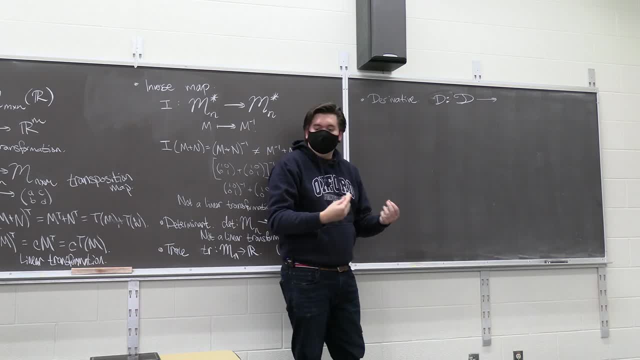 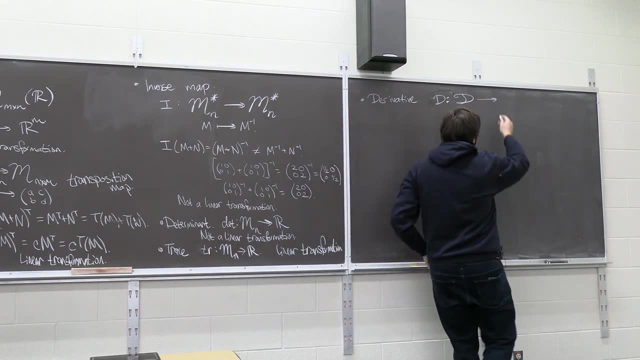 And what do you get out? Well, sometimes the derivative of a differentiable function is not itself differentiable. right, You can get like a weird derivative, but it's still going to be some nice, I don't know- say real value function. 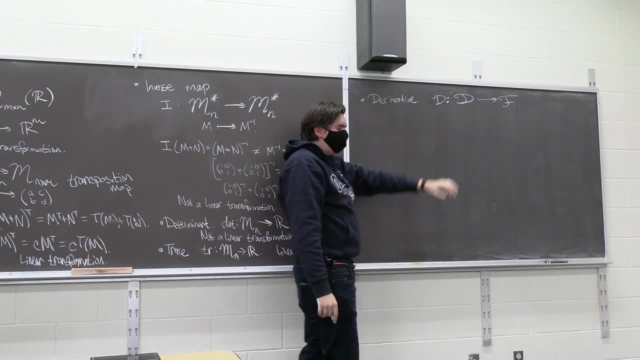 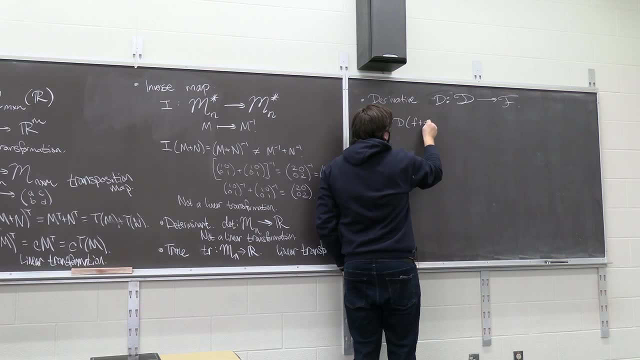 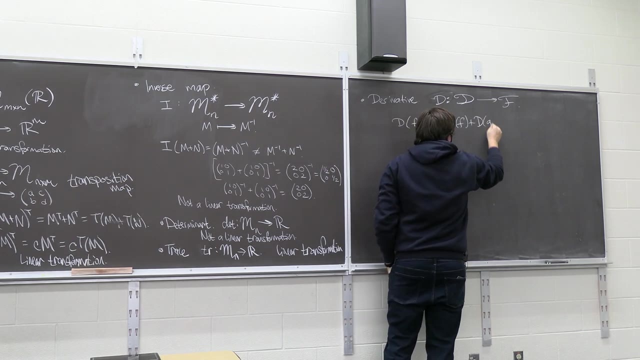 But you eat in some function that's differentiable and you get out some function. That's a map like that. Is it linear? What's the derivative of some function f plus some function g? It's just the derivative of f plus the derivative of g. 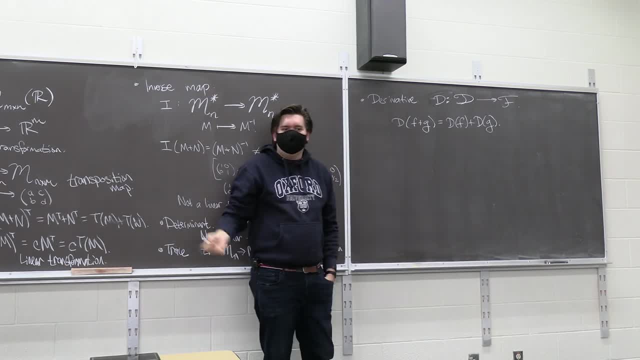 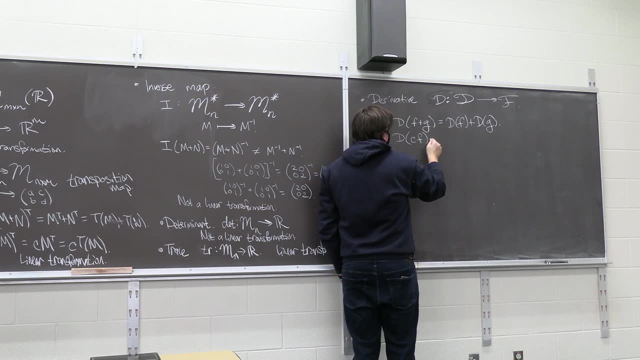 I mean this is like week three of single variable calculus or whatever, right, You have derivative properties And what's the derivative of some scalar times a function? You can pull the scalar out because you can pull it out of the limit, right? 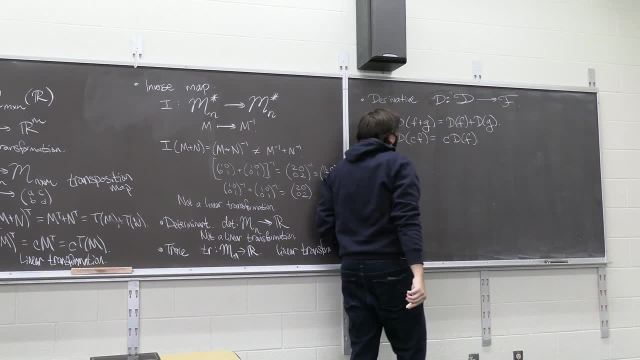 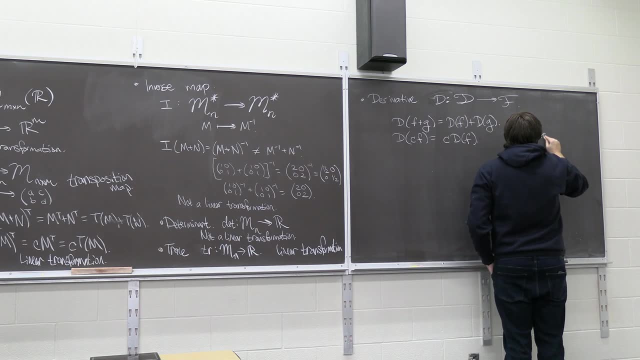 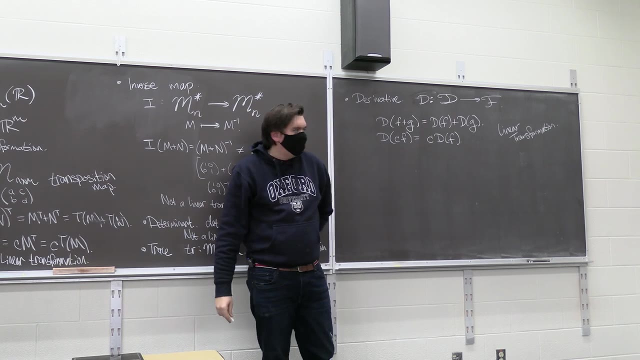 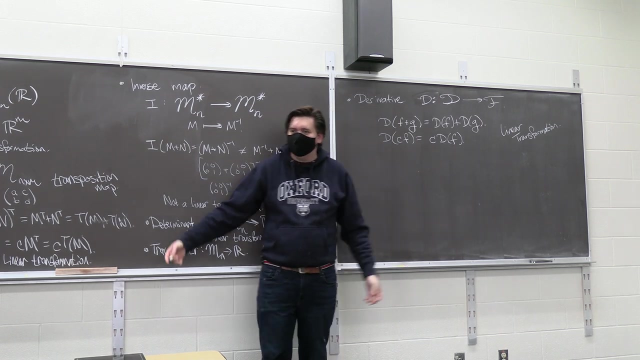 So it's just some scalar times, the derivative, So the derivative itself can be thought of as a linear transformation on a vector space, which is some collection of differentiable functions, And we could multiply examples. If it works for derivatives, well, maybe it works for integration also, right? 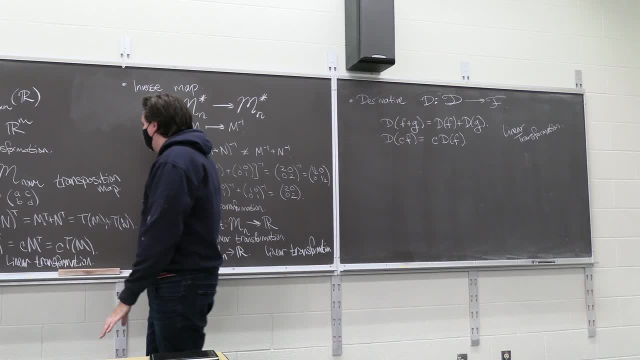 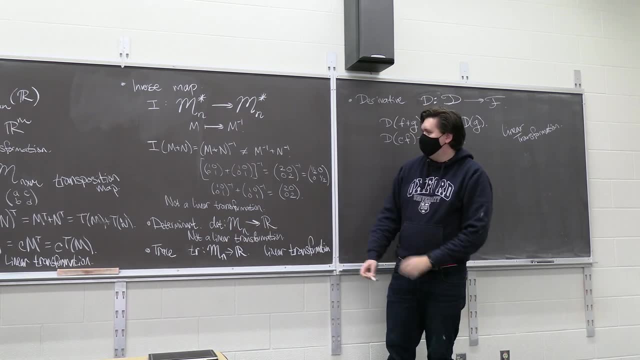 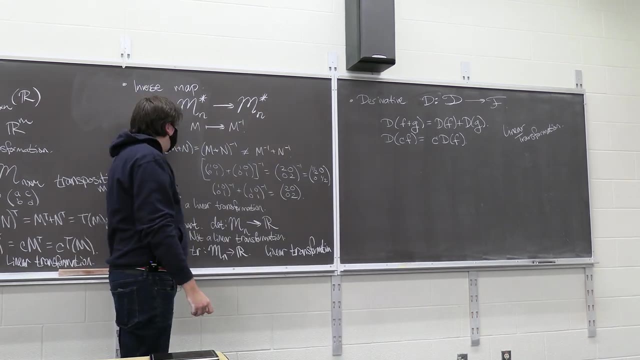 And so we can kind of think about all over the place. throughout your training up to this point, you've been seeing linear transformations as well as some things that are not quite linear. transformations like determinants, Great, Okay. Well, we started out by saying kind of a canonical example here. 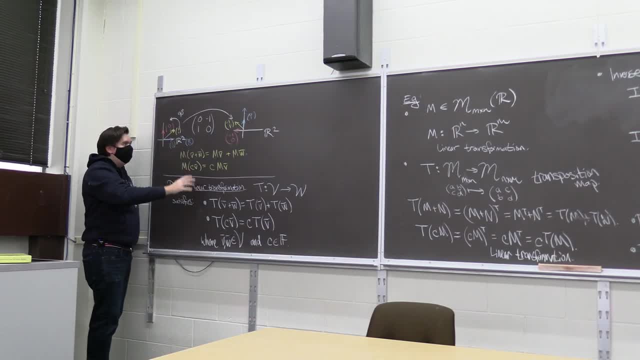 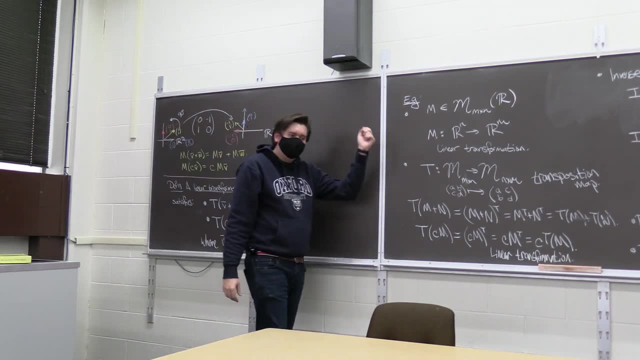 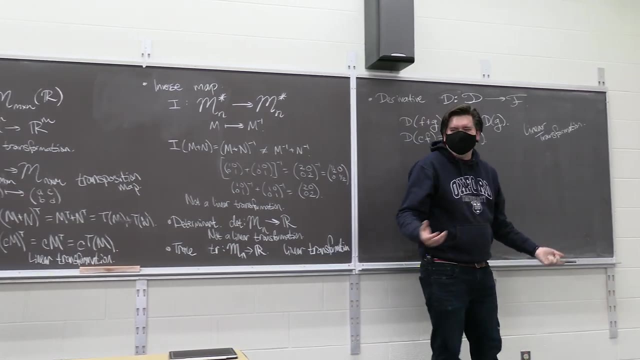 our motivation was a matrix, And we said matrices are secretly linear transformations. But then we went on to say, but there are lots of other things that are also linear transformations. Right, What we're going to say now is, yeah, but not really. 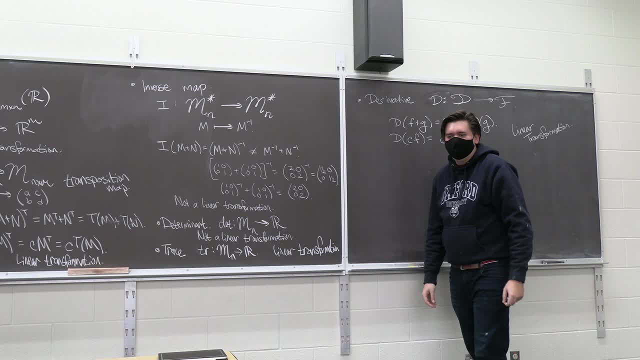 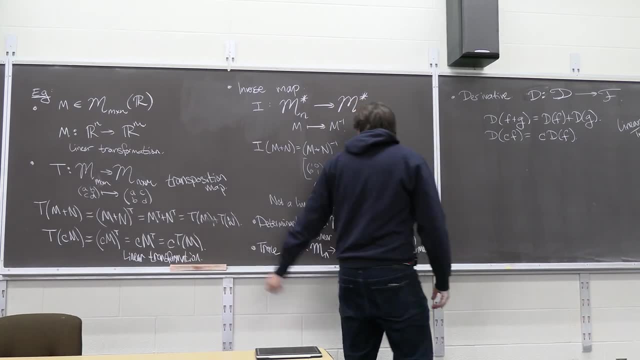 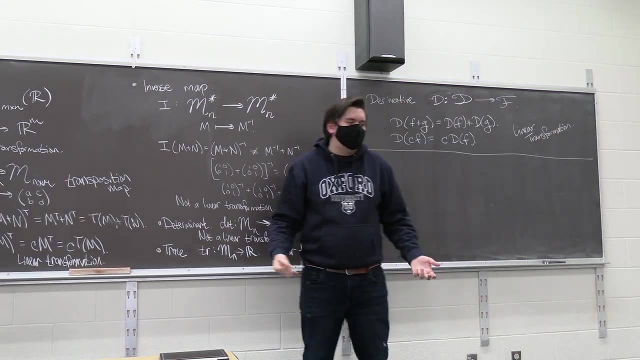 Actually all of these are matrices. I mean, this is why in linear algebra you pretty much just focus on matrices. It's like why don't you study all these other kinds of things? Because any linear transformation can be represented by a matrix. 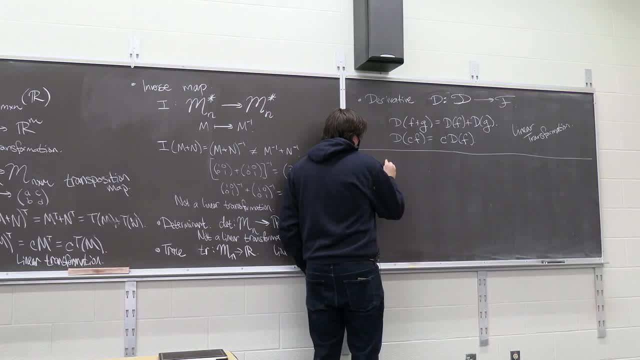 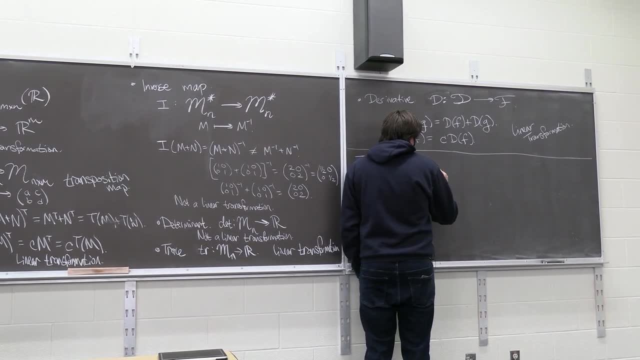 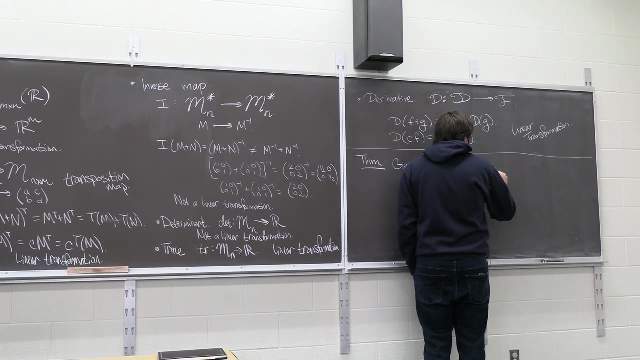 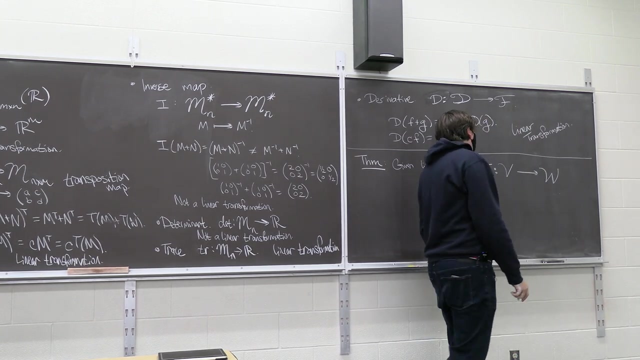 Let's make that precise. So here's our theorem that we want to show. If we're given some linear transformation- I'll call it T- from some vector space V to some vector space W, These vector spaces are going to have some basis. 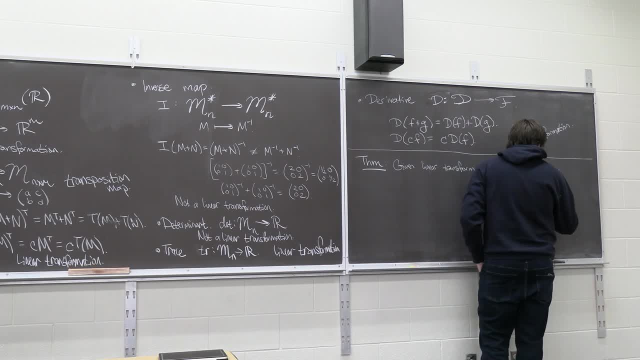 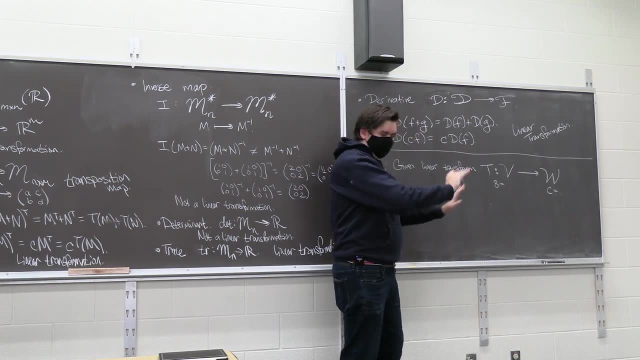 I'm going to call this one B. I'm going to call this one C, For today we're going to restrict our attention to finite basis. You might be wondering what if there's an infinite basis? We'll come back to those kinds of questions in a little while. 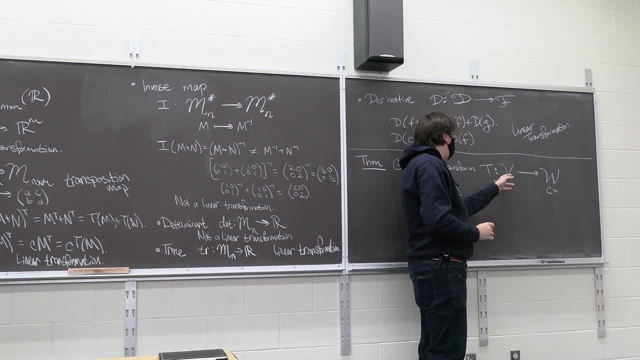 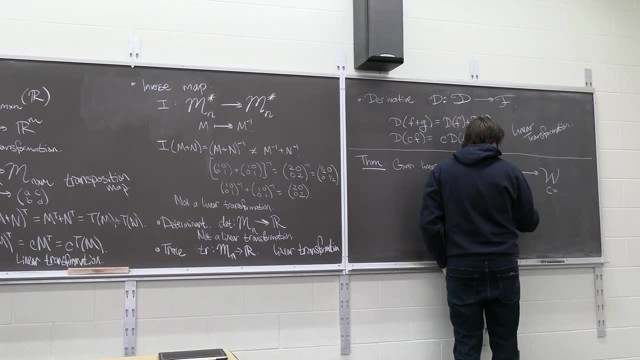 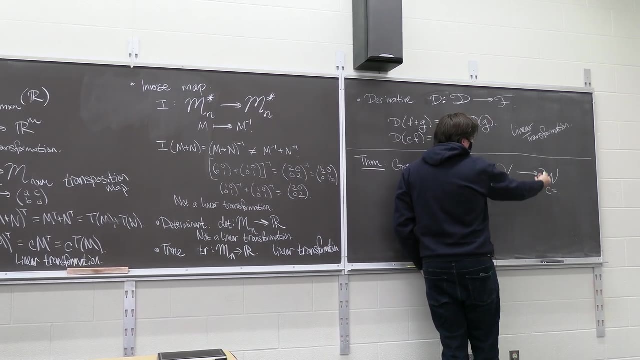 But for now let's say it's linear transformation from some finite dimensional vector space, some other finite dimensional vector space. So B has some basis, say comprising V1 through Vm. So this is an m-dimensional vector space. Let's say W is an n-dimensional vector space. 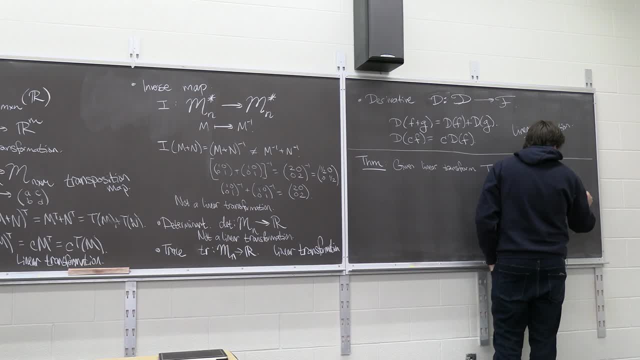 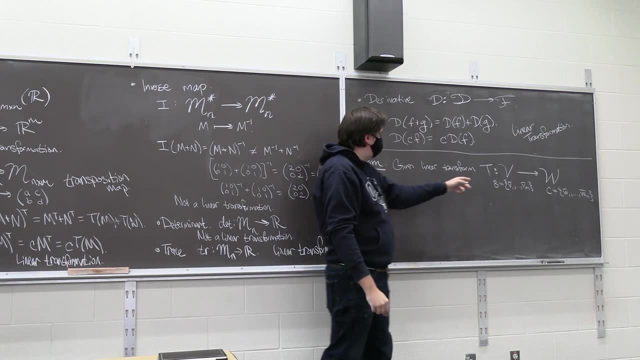 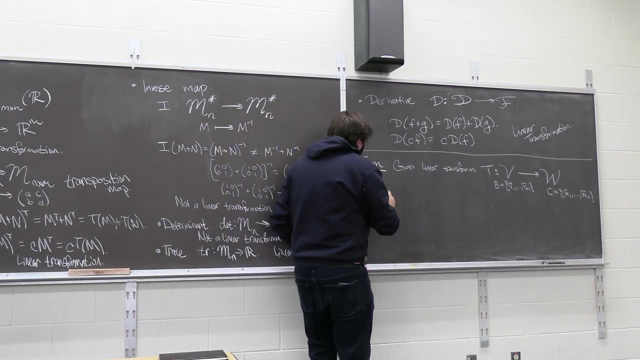 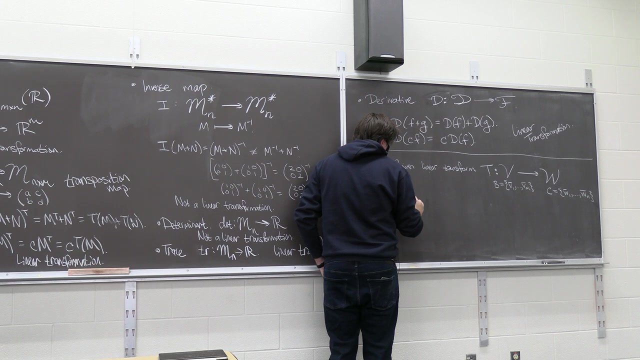 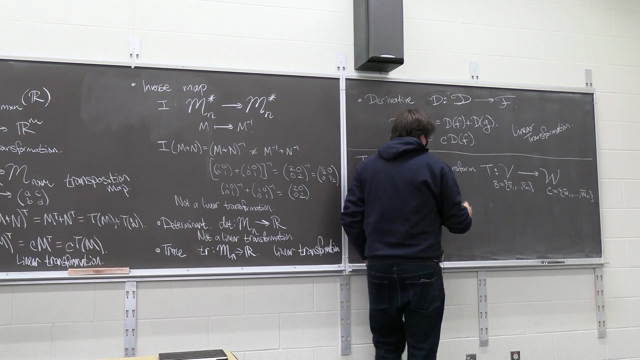 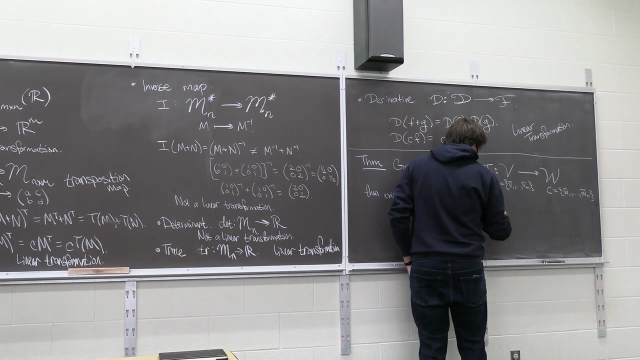 So it has some basis- W1 through Wn. Then what I want to say is: I can represent T by a matrix. So, more precisely, what I'm saying is that there exists a unique linear matrix which is going to be sending things in our basis in B. 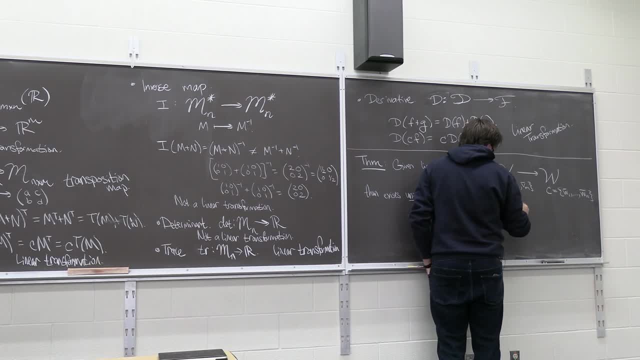 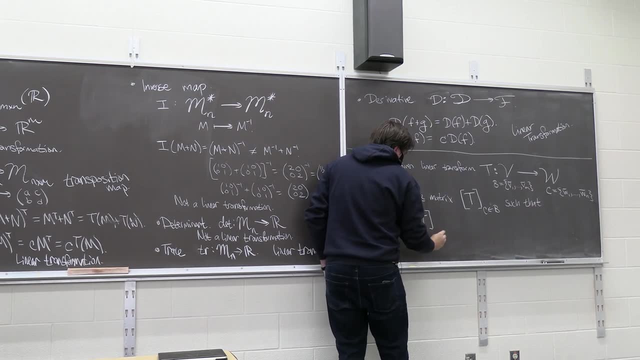 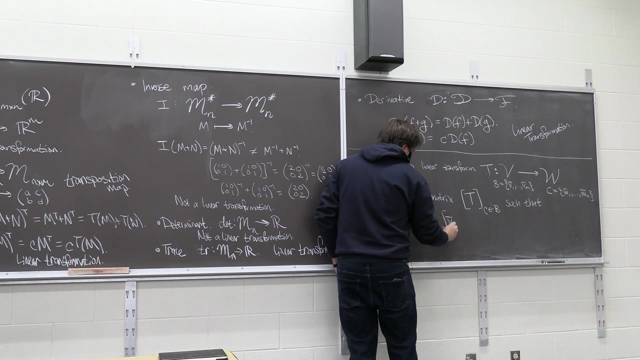 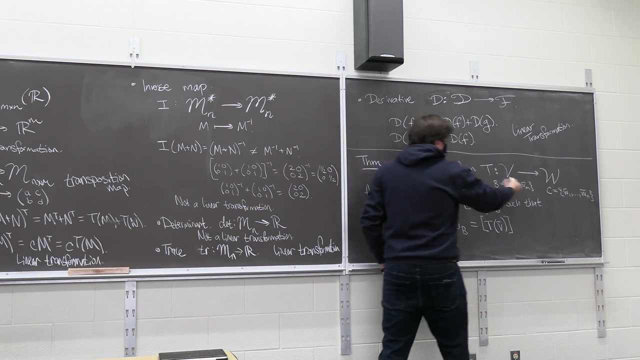 to things in our basis in C, such that that matrix times any vector in V expressed in terms of your basis B will send it to wherever the linear transformation T sends it, which is now going to live in W, so we can express that: 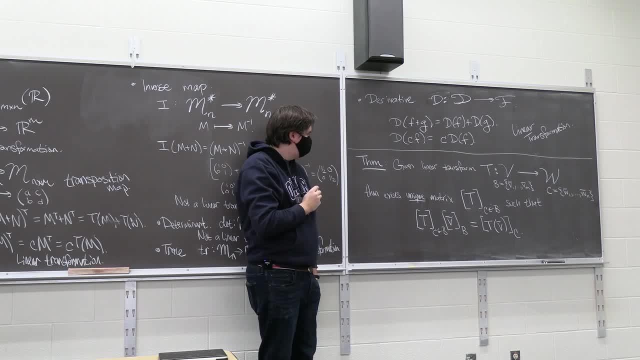 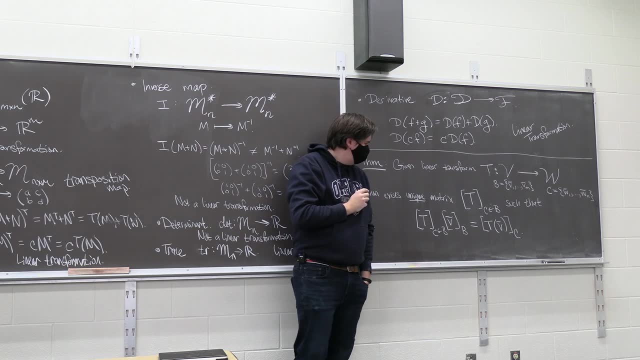 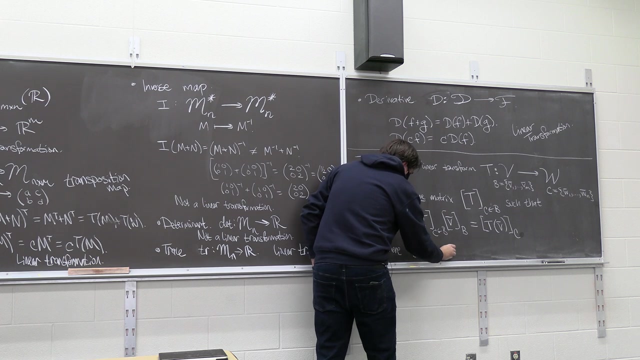 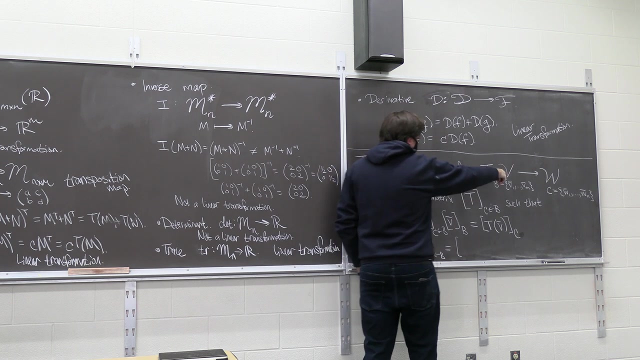 in terms of the basis C. Well, I should probably tell you what this matrix is, where that matrix can just be written as track, what your linear transformation does to each of your basis vectors of B. So what does T do to V1 through Vm? 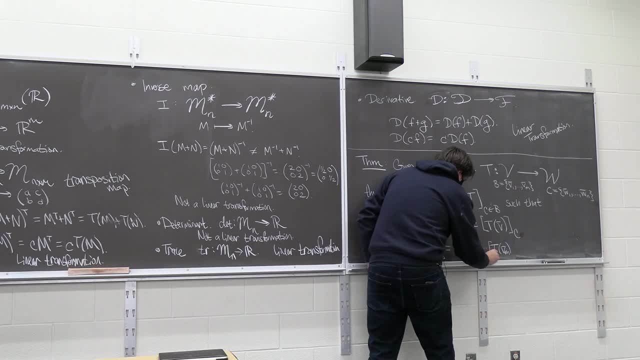 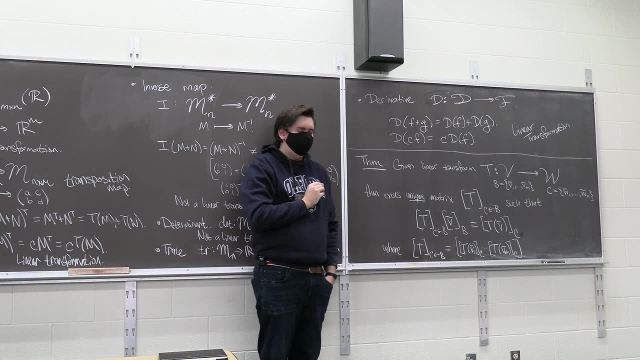 And then write those in terms of your basis, vector C. So maybe I'll give you a concrete example of this and then we'll come back and prove it. So for the concrete example, let's pick one of these guys. Oh, let's do this one, maybe. 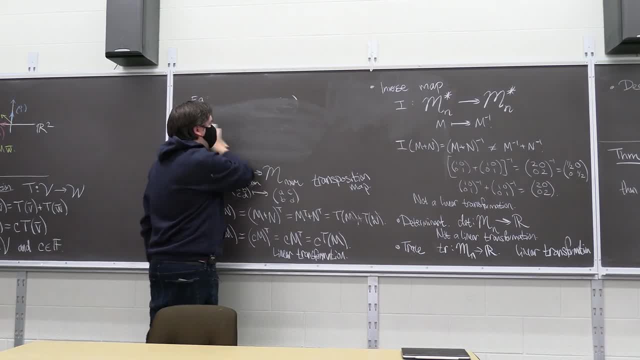 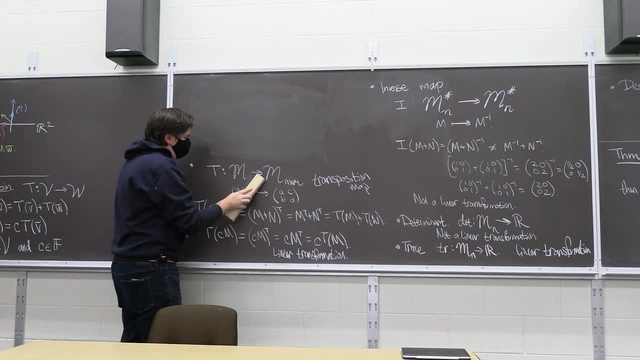 This linear transformation map? Can we, can we find? let me go back to the 2x2 case so it's a little more manageable. So let's say we have the linear transformation map, that's just the transposed map. 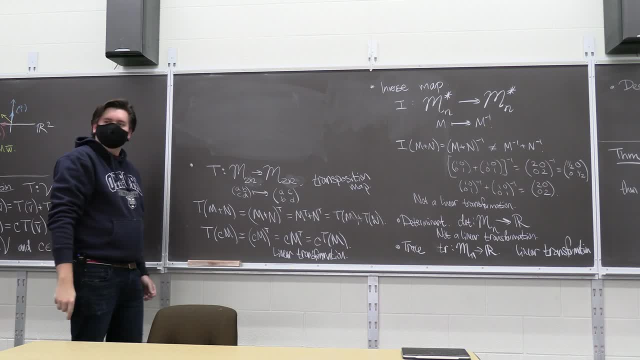 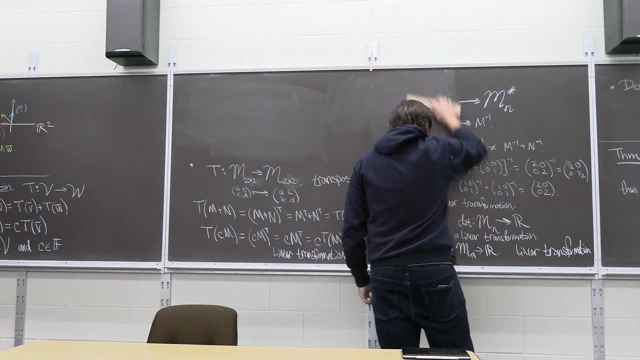 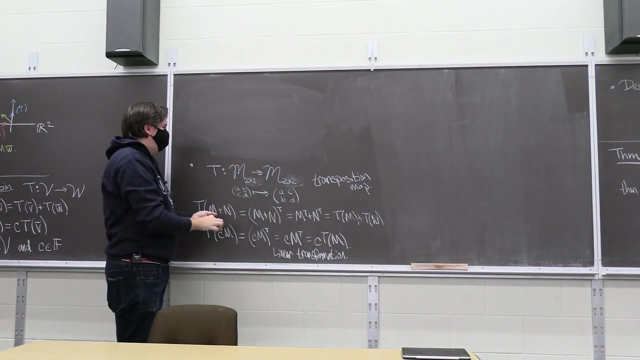 so transposition from 2x2 to 2x2.. Right, So let's think about this a little bit. Let me make some room for us to work. Well, what's a basis? What would our basis B be in this case? 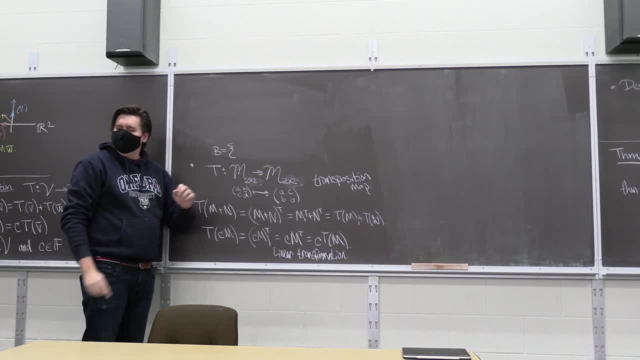 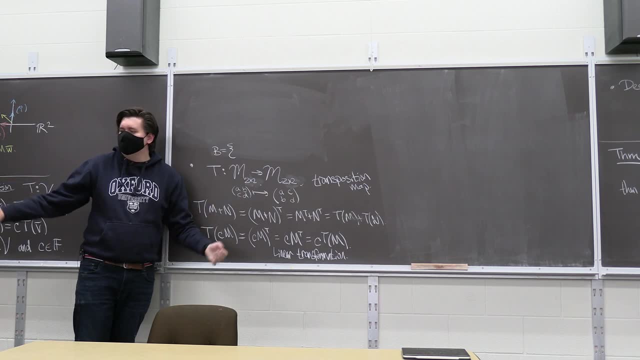 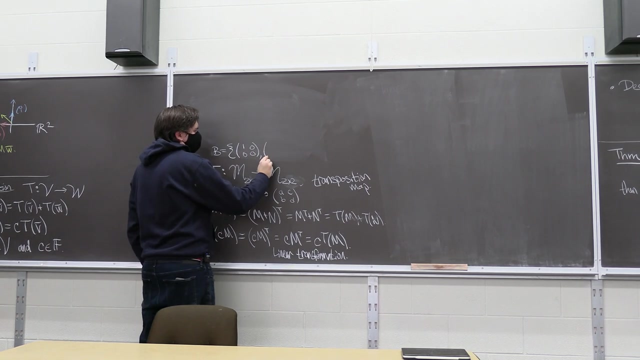 What's a basis for the collection of 2x2 matrices, Assuming like we're working over real scalars or whatever? What's a very natural basis? Yeah, one in like the top left corner and then you can have like a one. 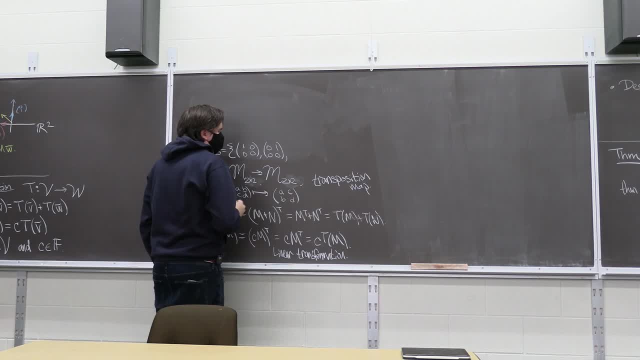 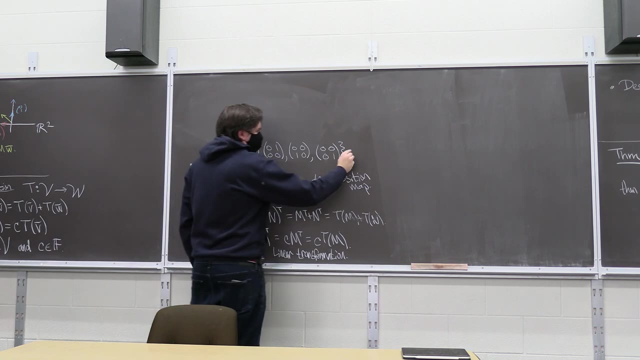 say in the top right corner, and then you can have one in like the bottom left corner and one in the bottom right corner, And since it's a map from its vector space to itself, we'll also have that be our basis for the second guy. 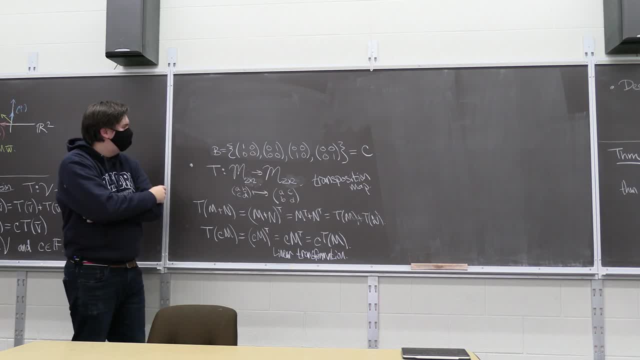 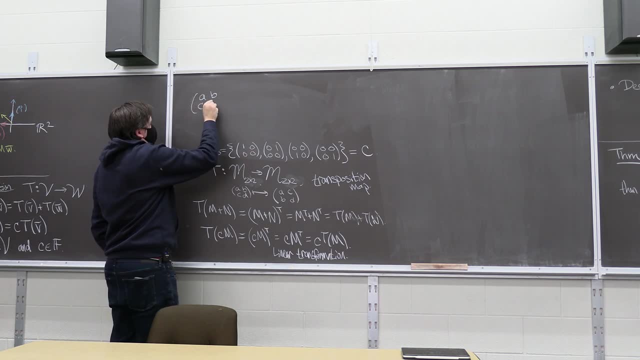 Right, So both our bases will be in terms of this guy. So like, just remember how this works: If I have some matrix here, like some matrix A, B, C, D, and I want to express it in terms of this basis, 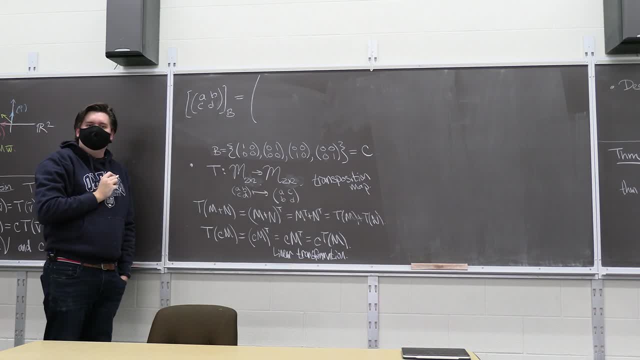 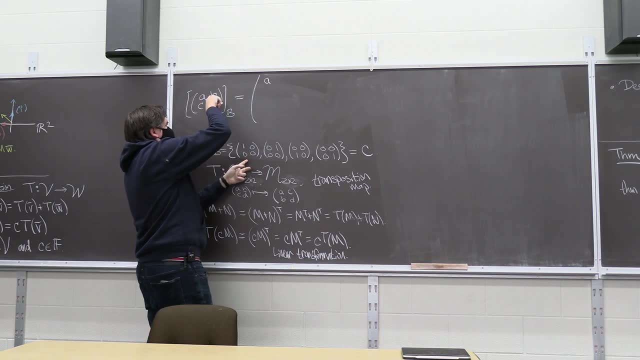 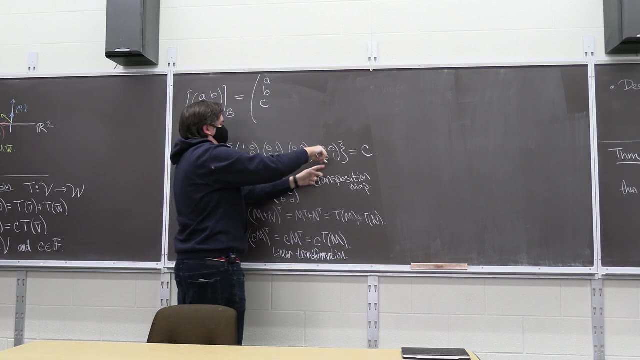 what will that give me? What vector? Well, like this is just going to be: A copies of the first element plus B copies of the second in your basis, plus C copies of your third basis element, plus four copies of D copies of your fourth basis element. 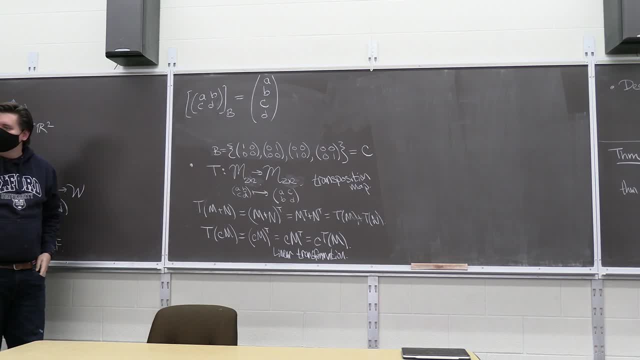 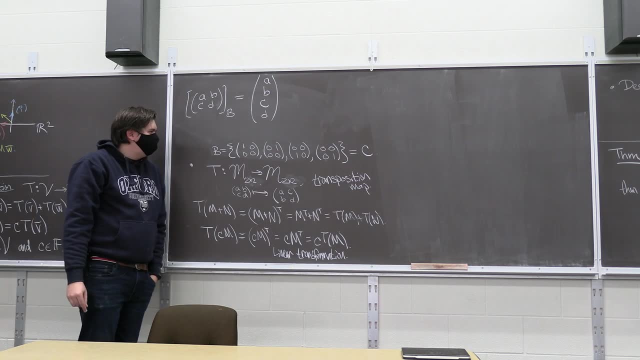 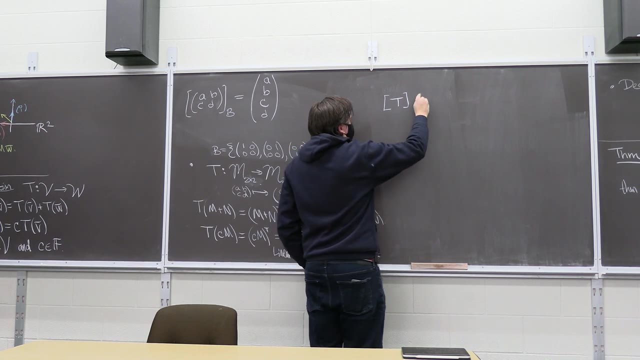 Right, So that's just that vector. Okay. well, the claim is: in order for us to see what this matrix is like, what is the matrix that corresponds to T, that that matrix is just? I'm not going to write the basis here. 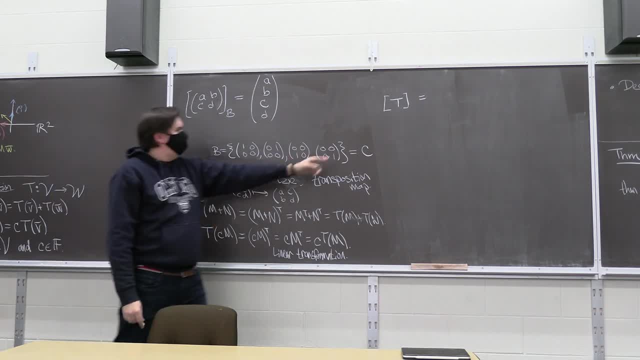 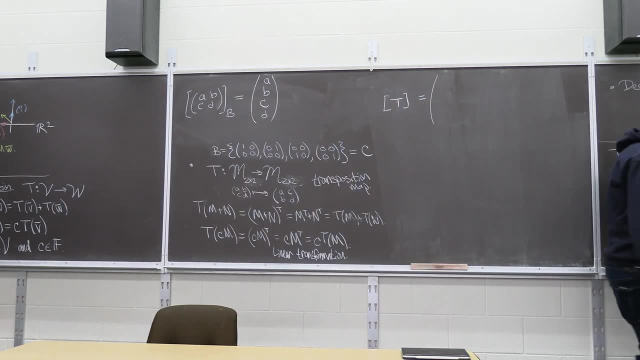 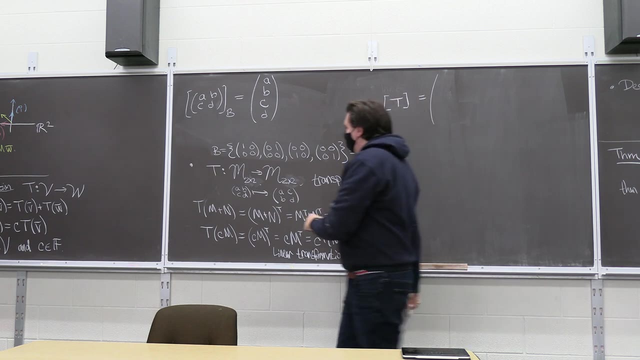 because it's just one basis we're working with. so it's pretty obvious. But the matrix corresponding to T we find by. just for each column we say what happens to your first basis vector all the way through your last basis vector. Okay, so what happens to your first basis vector? 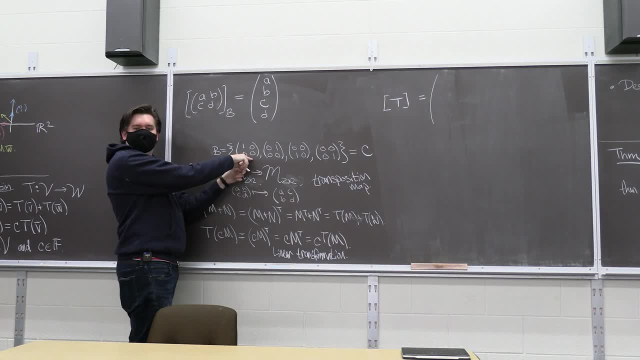 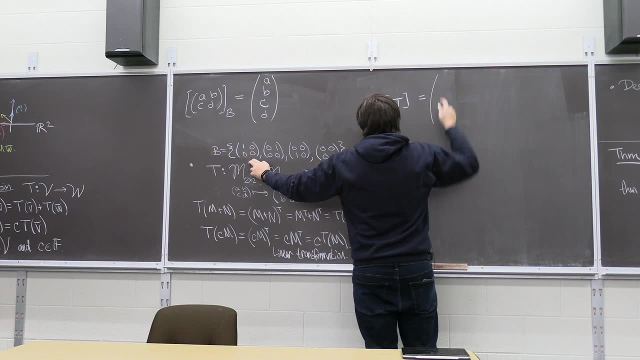 Will the transpose due to this guy? Leaves are the same right, So we'll write in coordinates. this is the thing responding to the image of one zero, zero one which is itself one zero, zero one. 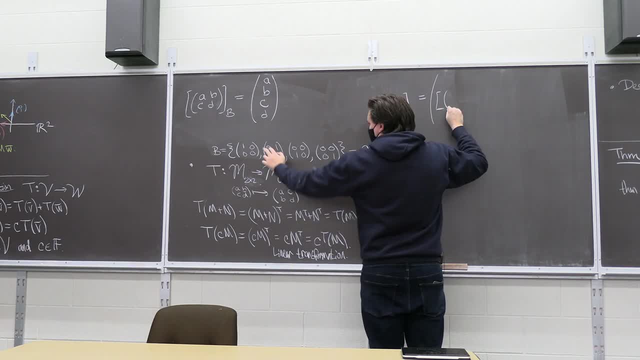 Well, let me do it in two steps. So the image of this, the transpose of this, is just one: zero, zero, zero. And then for your next column you're like: well, what is the transpose? due to this guy? 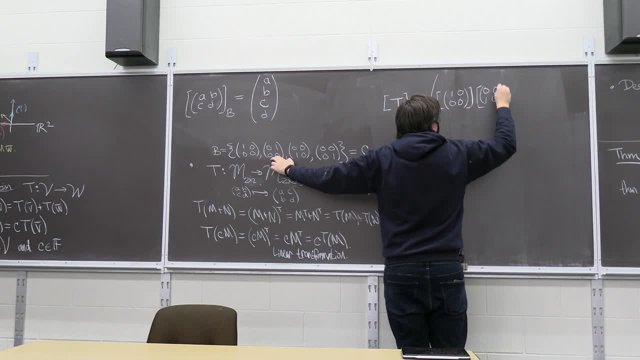 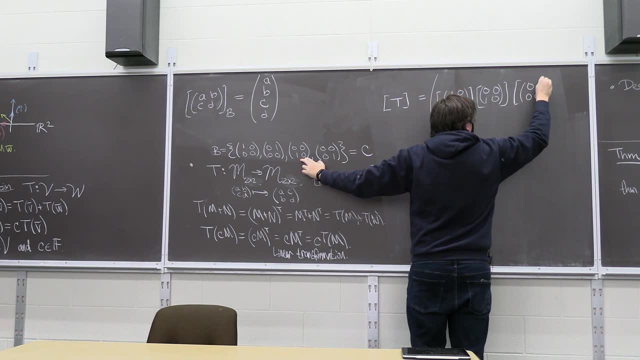 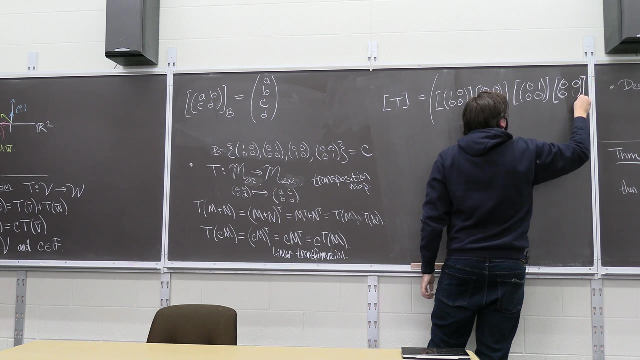 Yeah, he's just going to get changed into something like this. And then for the next one, you're like: well, this just gets changed into something like this, And the last one stays the same. And now, in terms of our coordinates, 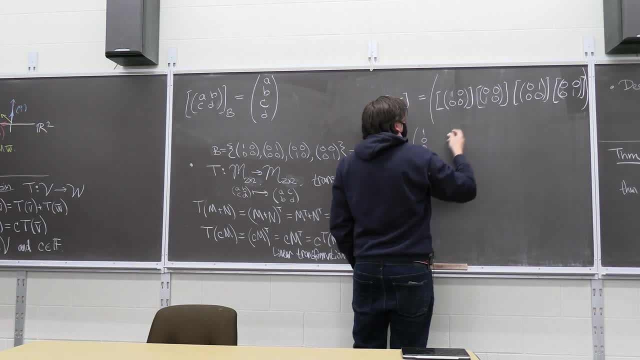 this will just give us one zero, zero, zero. The second guy is zero, zero, one, zero. This next guy is zero, one, zero, zero. And the last one is zero, zero, zero, one. Yeah. 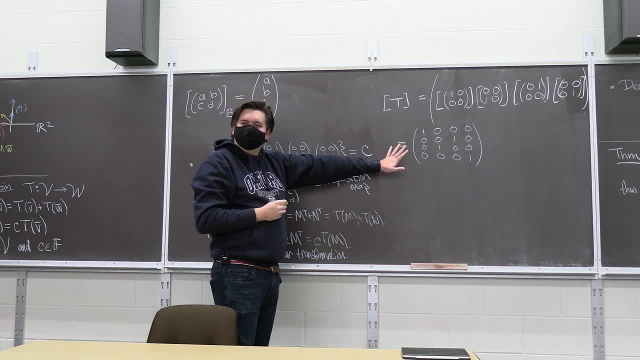 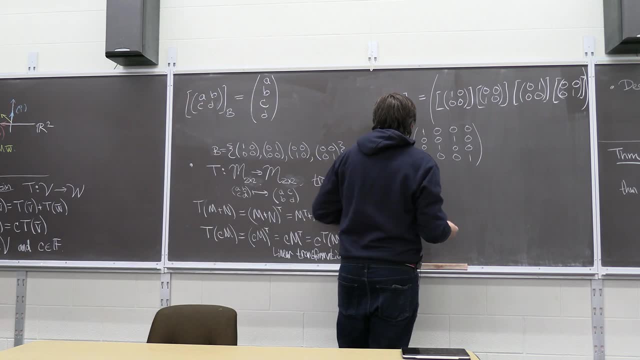 So the claim is: that is our matrix, And so like, let's double check Right, Like, if I want to know, like, what is my transformation due to something like A, B, C, D. well, the claim is: this should really 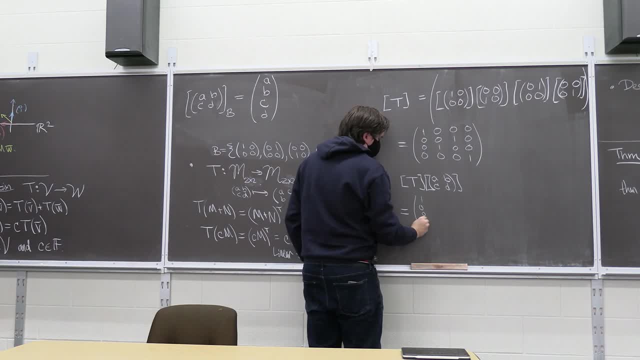 well, what's going to come out Like? it's going to be this matrix: one zero, zero, zero, zero, zero, one, zero, zero, one, zero, zero, Zero, zero, zero one. 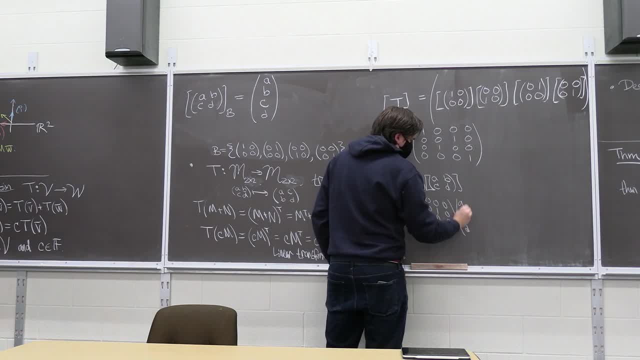 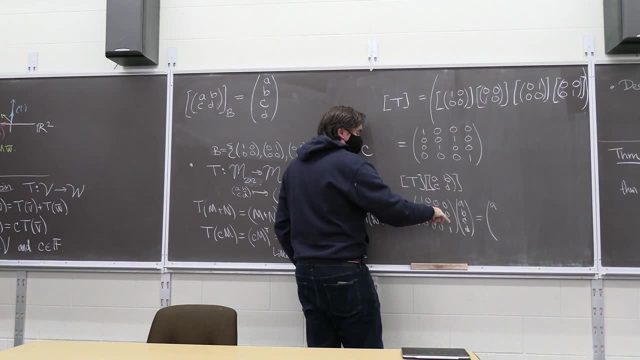 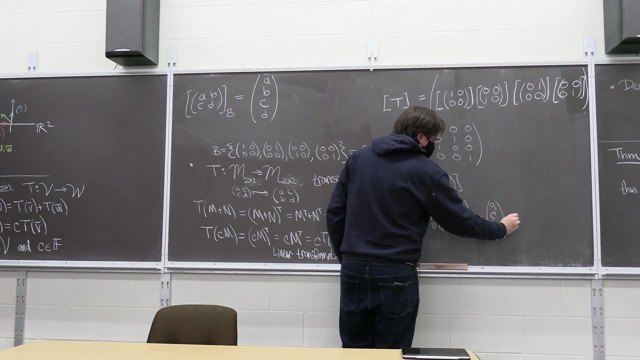 It's like: what is that going to do to the vector A, B, C, D? And you're like, well, when you multiply this, you're going to get out A and then C, and then B and then D. 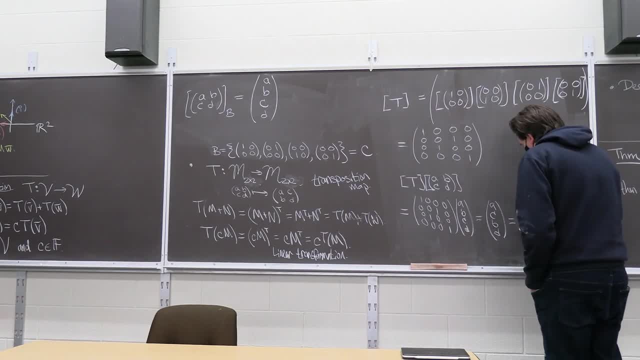 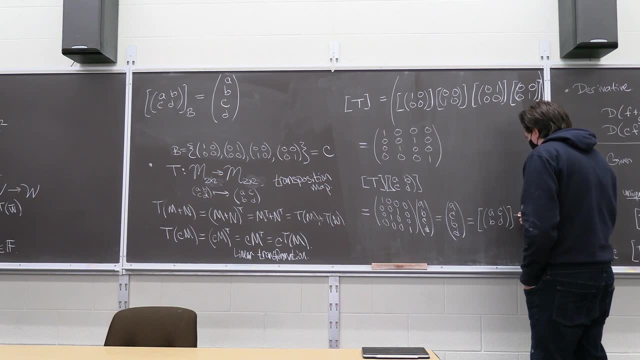 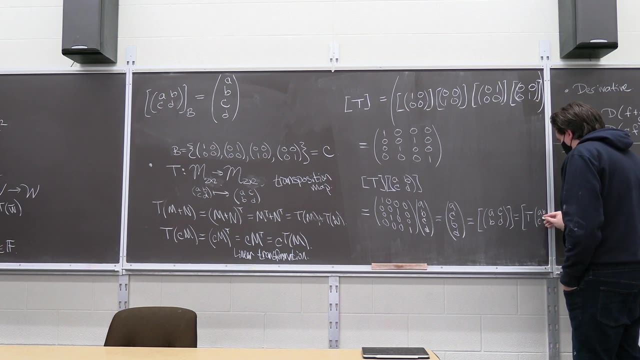 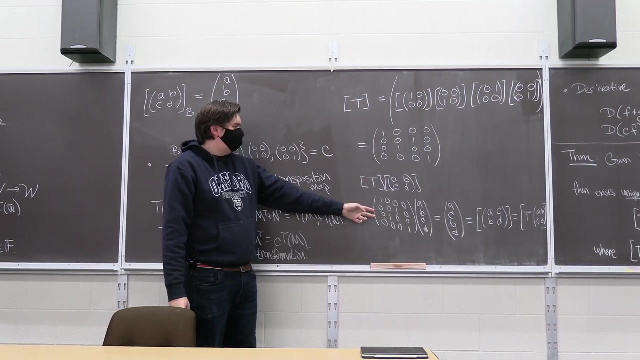 which is exactly the coordinate representation of the vector A, C, B, D, Which, sure enough, is the transpose of the original matrix A, B, C, D. So multiplying by this matrix accomplished the same thing as taking a transpose. 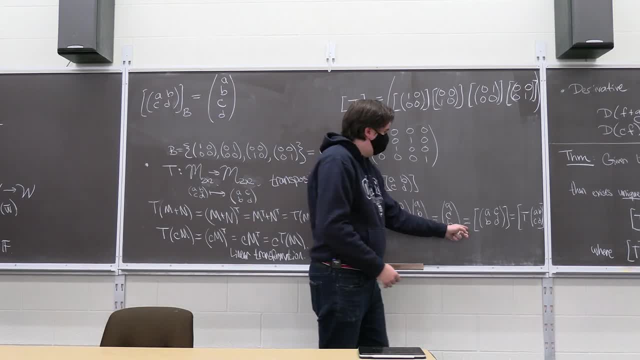 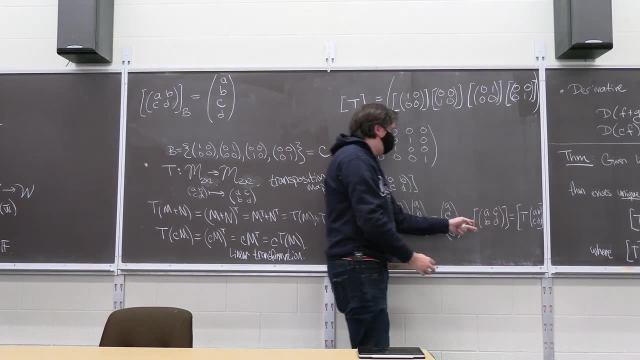 Like this step. this is saying the coordinate vector corresponding to this matrix. And what is the coordinate vector corresponding to this matrix? Well, in terms of your basis. so here I'm doing it in terms of I'm not writing B every time. 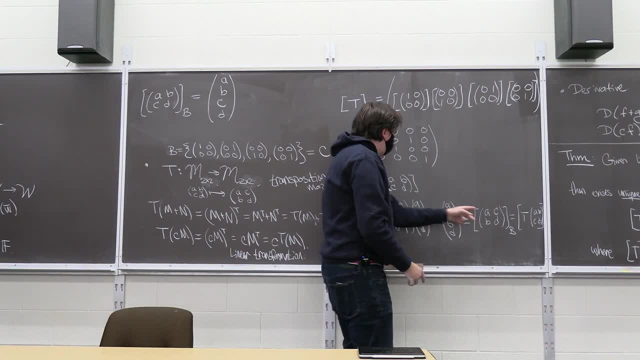 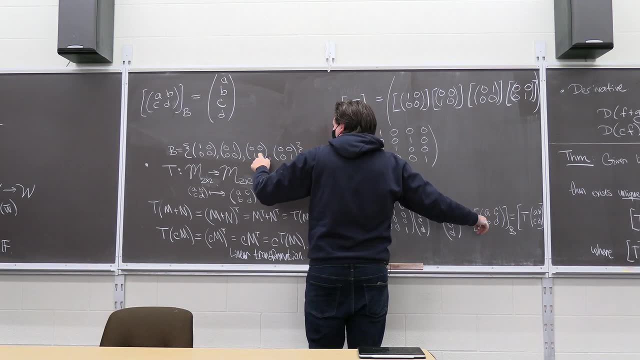 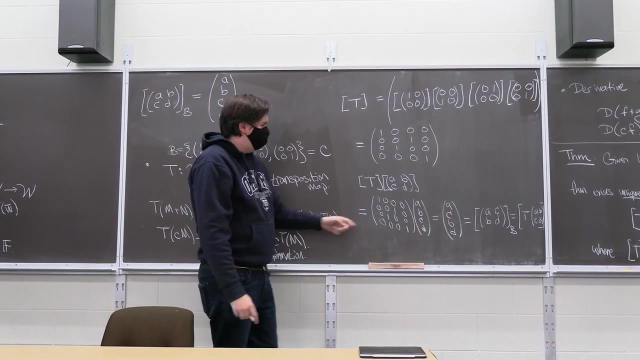 but it's in terms of my basis B. This is just A copies of the first one, C copies of the second, B copies of the third and D copies of the fourth, which is exactly what that's saying In coordinates. So that's just reading off the coordinates. 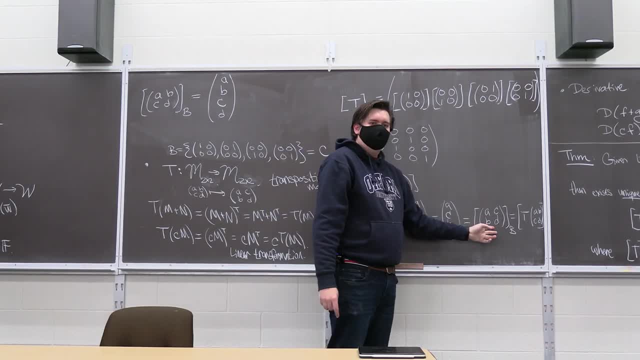 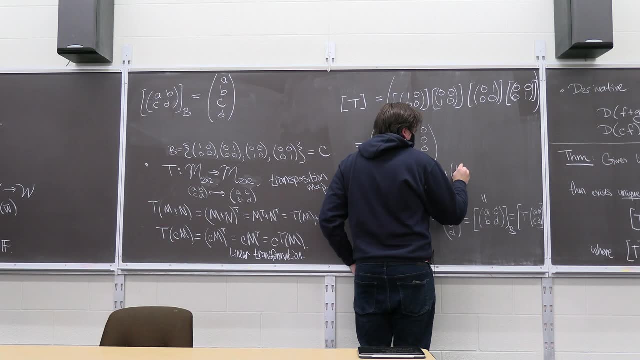 in terms of our basis B to build this guy That is. this is just a linear combination in terms of: B of A- copies of your first basis vector plus B copies of your next basis. C- copies of your next basis vector plus B copies of your next basis vector. 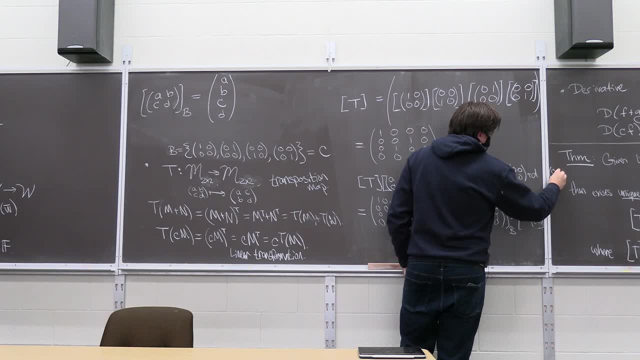 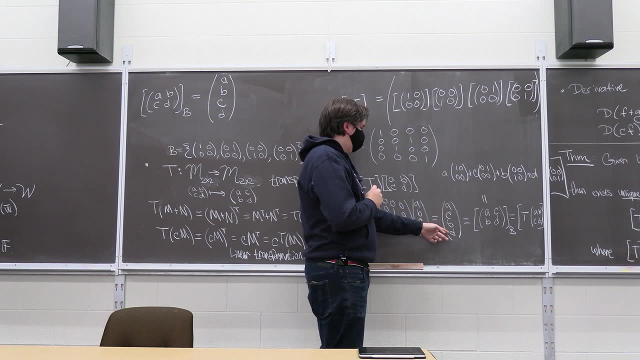 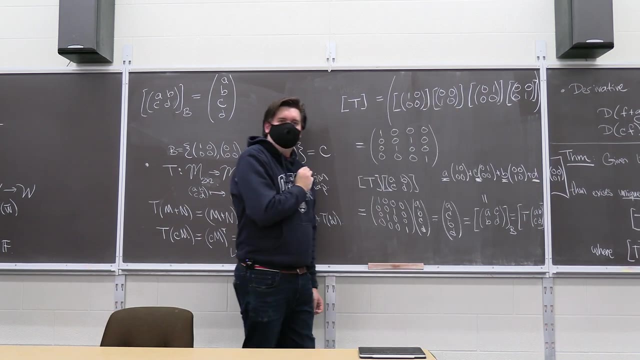 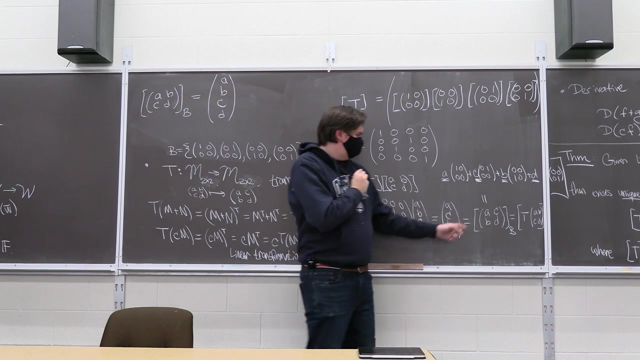 plus D copies of your next basis vector, plus B copies of your last basis vector. And so this is the vector, the coordinate vector. that's just listing these coordinates. So these square parentheses are just me asking what is the coordinate vector corresponding to this matrix? 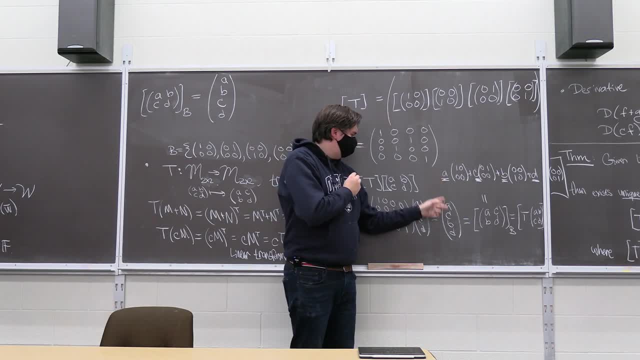 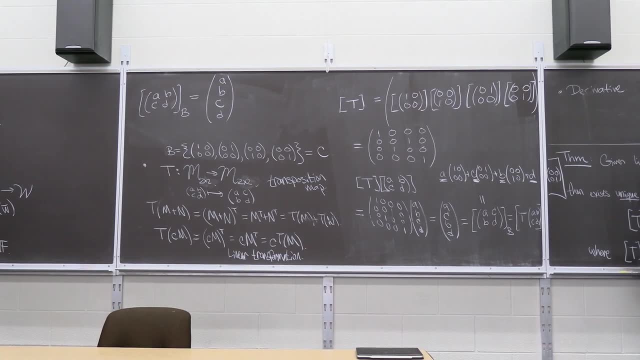 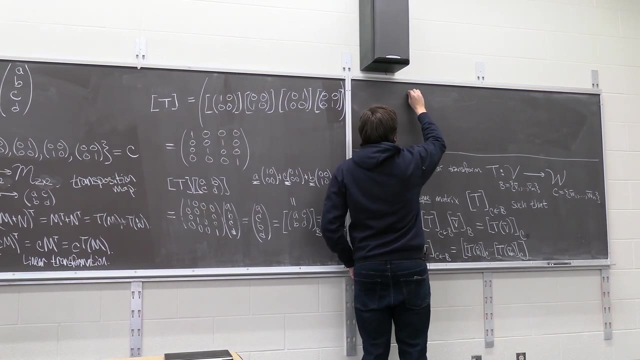 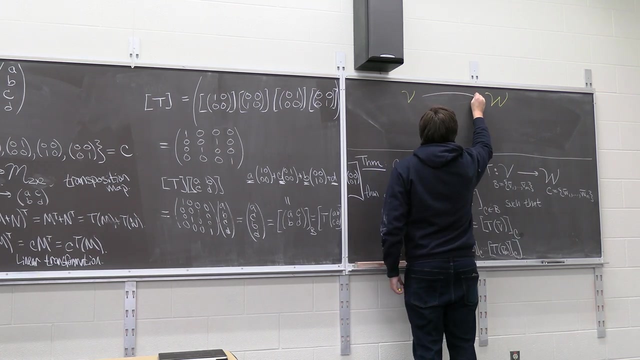 In terms of the basis B, And it is precisely this coordinate vector, So maybe a picture is helpful here. A linear transformation is some map that's happening up here from some V to some W, So a linear transformation T is taking place up here. 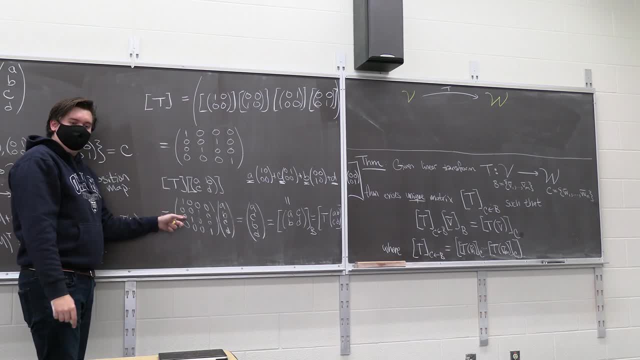 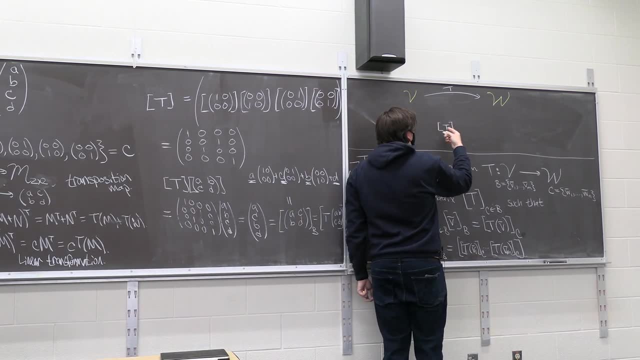 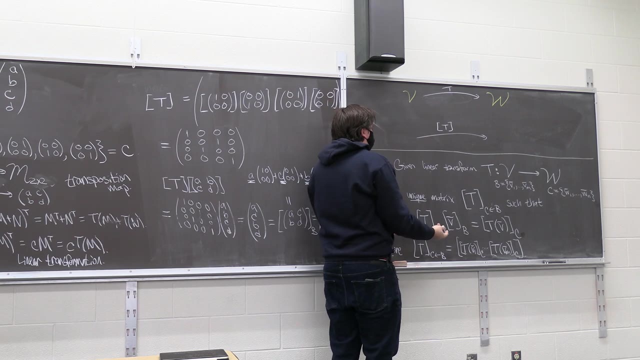 What? this box around T, the matrix, that's not happening up there. This box around T is a matrix And it's happening down here between the vector spaces you get by the you're looking at. oh, what are the coefficients of my basis B? 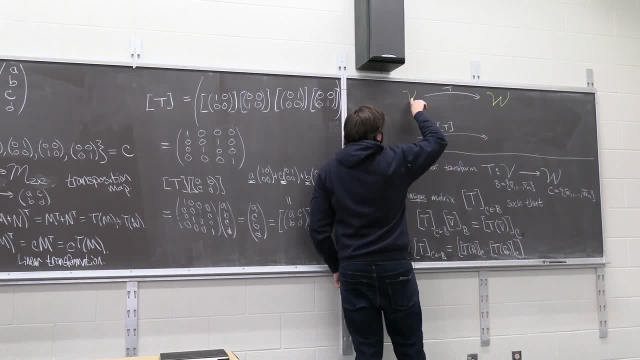 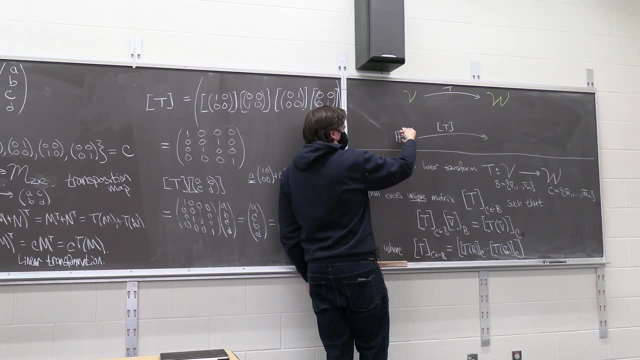 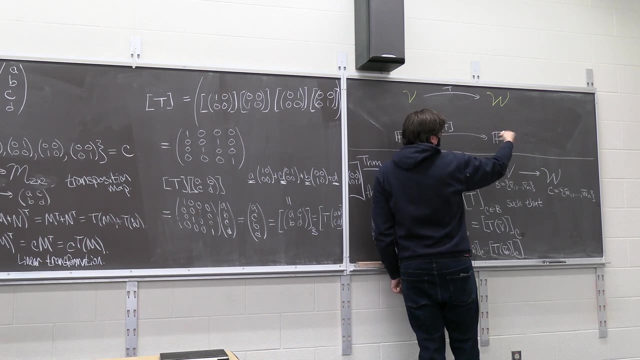 and my basis C. So you're like: well, if V is M dimensional, this is like R to the M or, more generally, F to the M, And if W is N dimensional, this is whatever you feel, like R to the or C, whatever your field is. 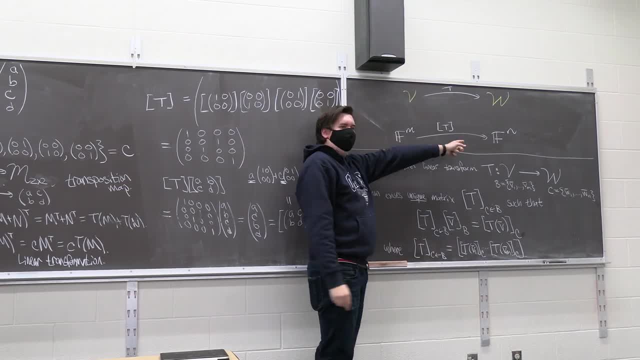 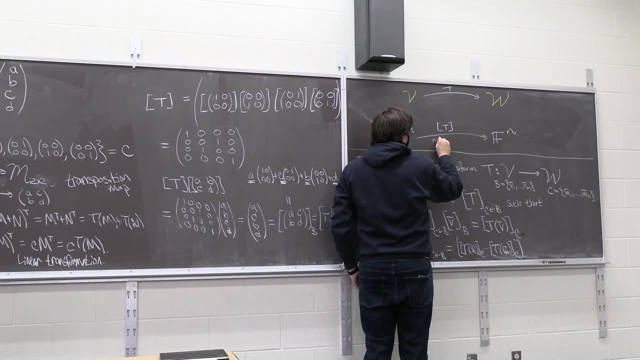 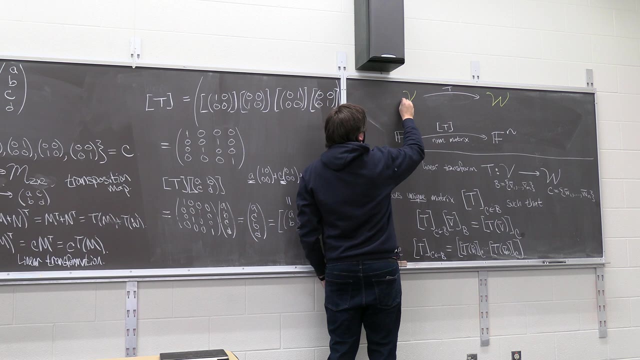 to the N. These are your coefficients. This here is a N by M matrix, And so what we do is, when you have some vector up here, some vector V, that vector gets sent down by looking at what is vector in terms of some basis B. 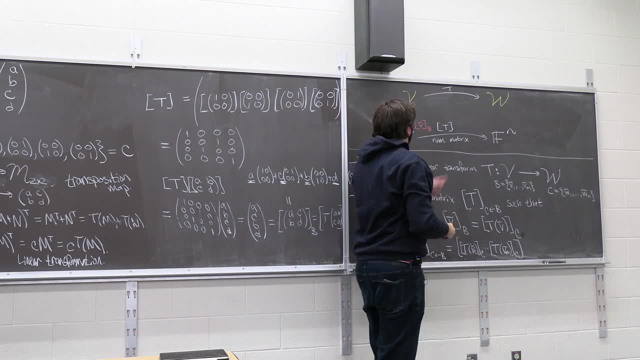 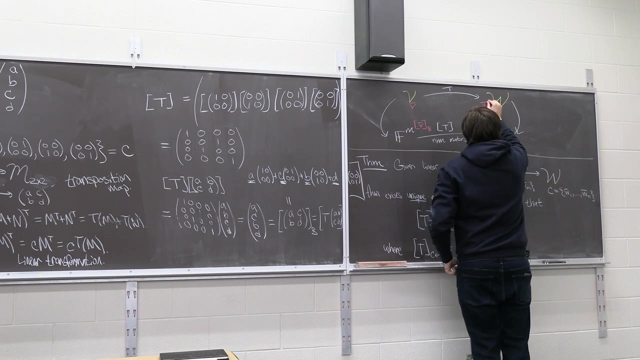 And then we send it over here by this map And you're going to get some resulting vector in terms of your basis for C. So it's like same thing: here There's some, there's a map you can think about that sends vectors W. 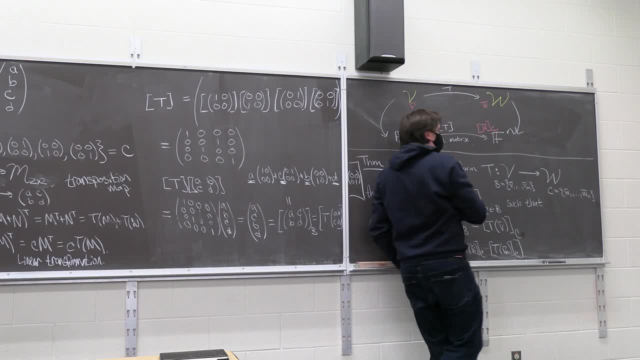 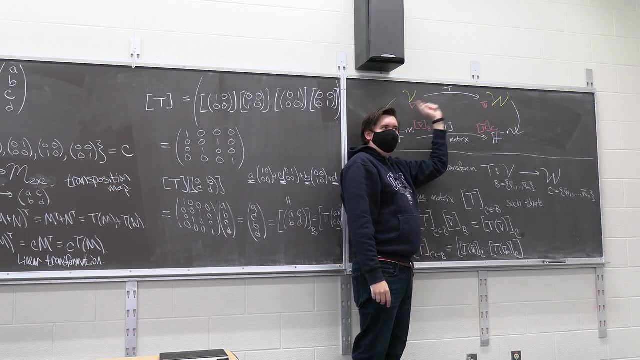 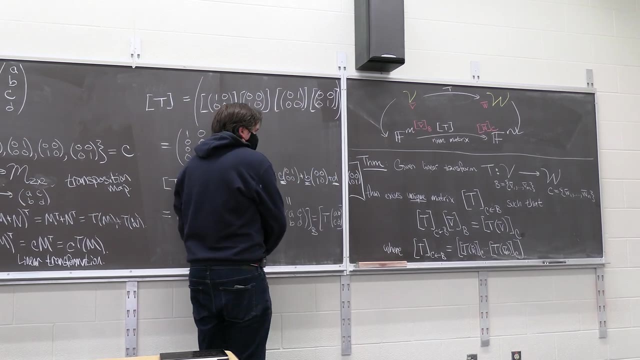 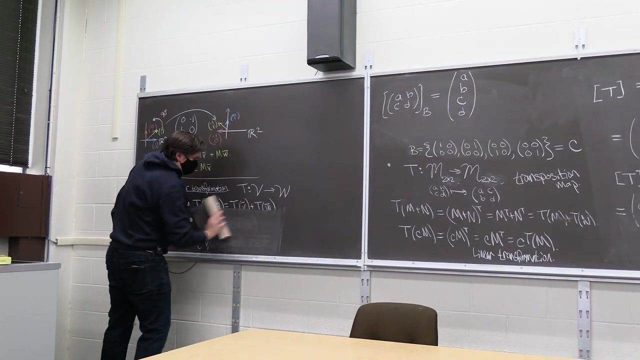 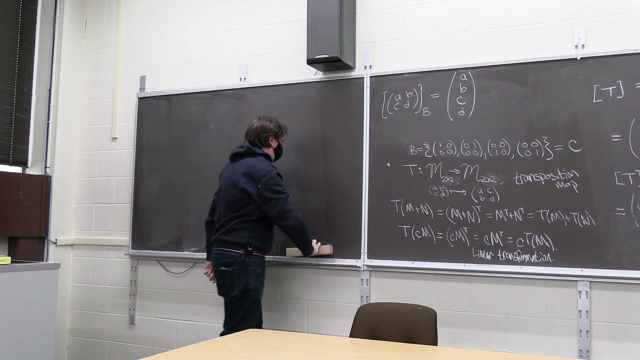 down to those vectors in terms of the basis C. So the matrix is representing down here the linear transformation that's taking place up there. Okay, We have very little time left, So let's go ahead and prove this. So I want to show. 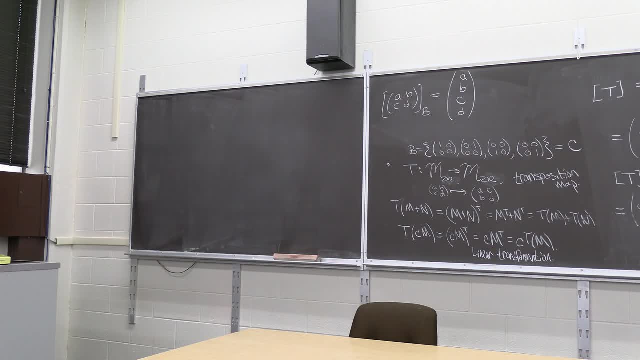 that the matrix that does this, that this matrix does this and that it's unique. There's two parts to it. So first let me show that this matrix actually does this. So I want to prove the theorem now. So I have V. 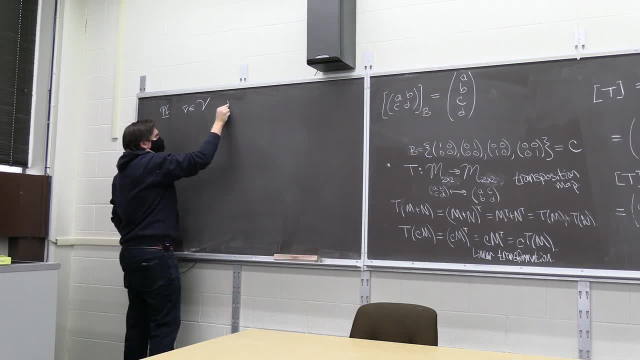 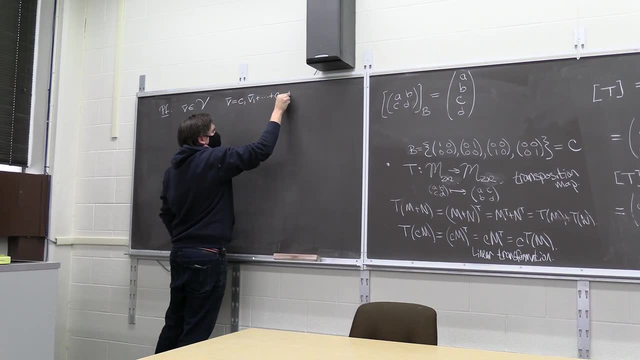 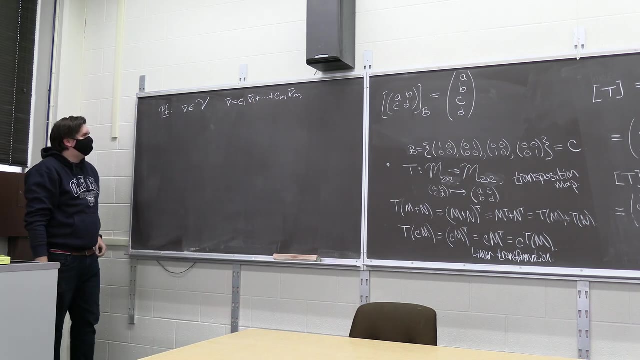 as some element of my vector space. So I can write V as some number of copies of V1 through some number of copies of Vm, where these are my basis vectors for my basis B, my basis for the vector space. And now I want to ask: 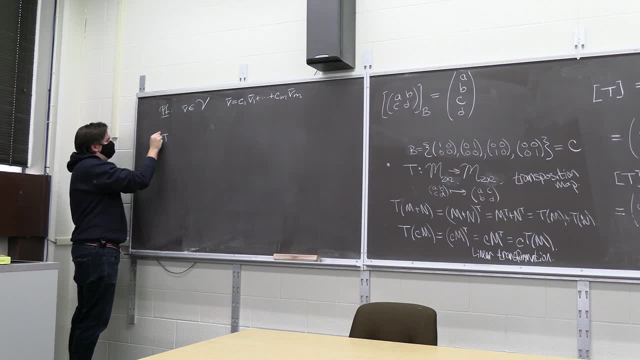 what does? what does this matrix times V give me? Where this is, the V is expressed in terms of the basis B and this is a map from B to C, B to C, And we just said: well, this matrix. 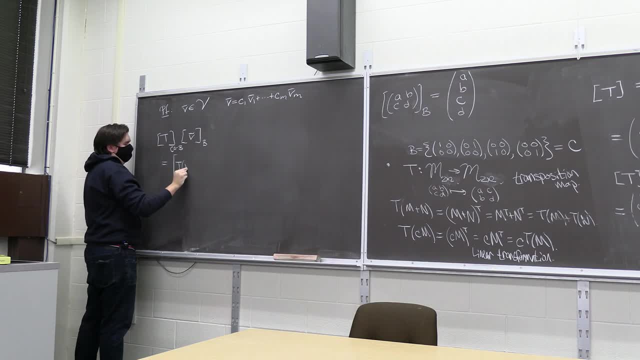 we want to redefine it to be T of V1 through T of Vm, all written in terms of your C basis, where C is a basis for the vector space, W times your vector V. But what is the vector V in terms of the basis B? 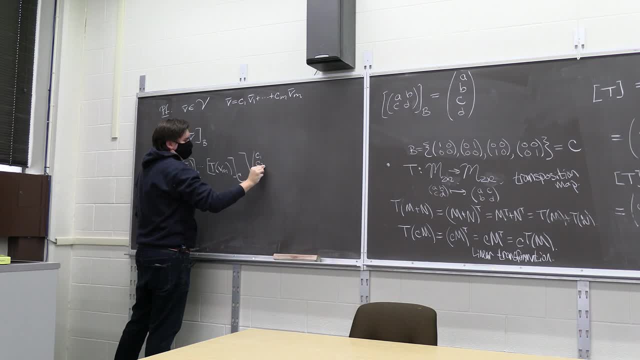 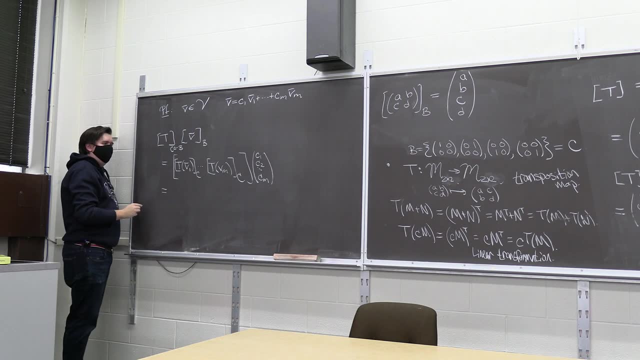 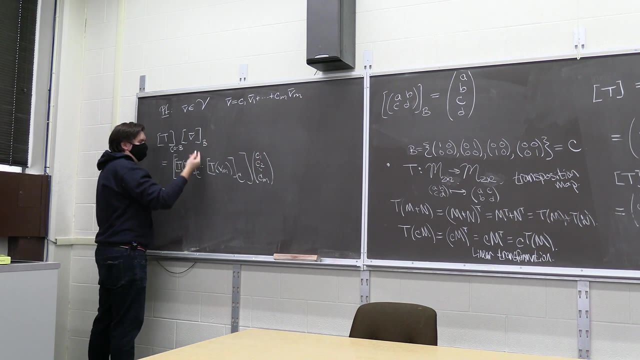 It's just your coordinates C1,, C2, through Cm. Remember, when you multiply a matrix by a vector, it's just the first value times the first column, the second value times the second column, all the way through the third. 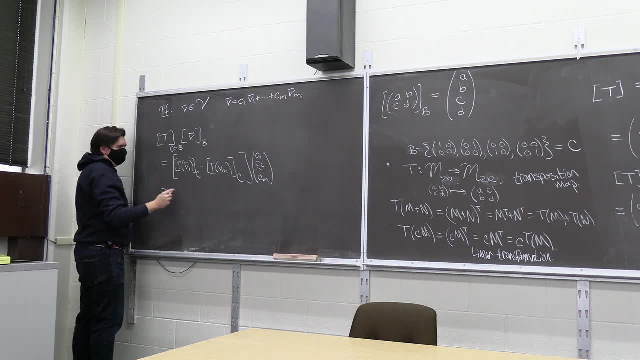 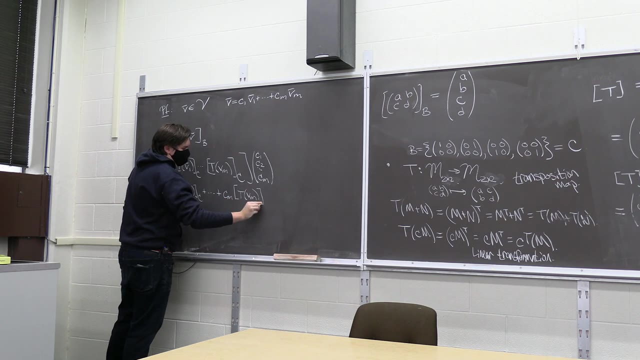 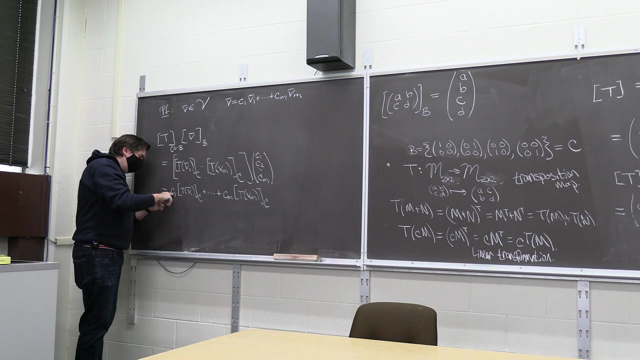 fourth, fifth, through the last times, the last column. So this will just be C1 copies of the first column through Cm copies of the last column. But scaling the coordinate vector is the same as the coordinate vector of the scaled vector. 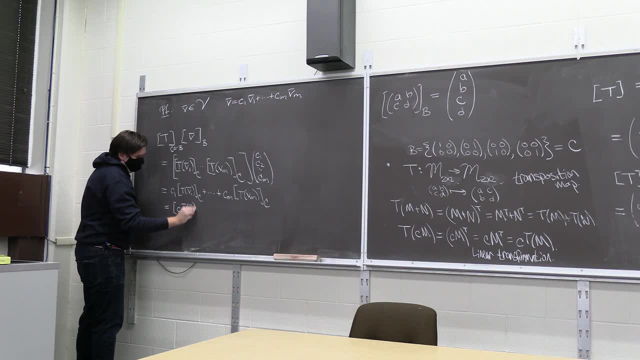 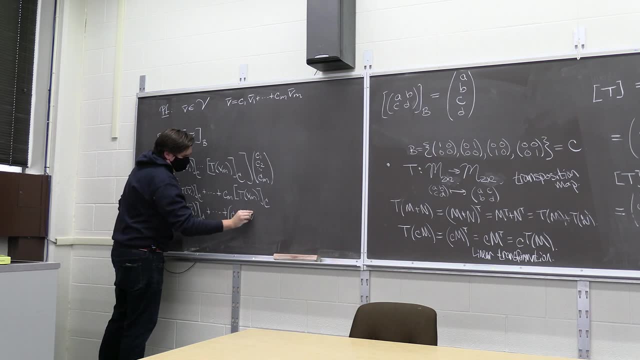 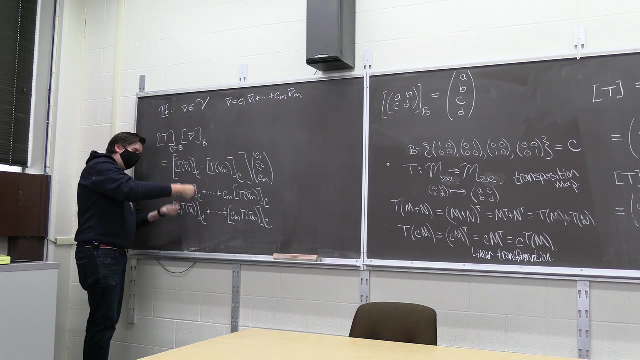 That is, we can bring these inside And the coordinate vector of a sum of vectors is the same as the sum of the coordinate vectors, That is, this is the same thing as just C1, T, V1 through Cm, T, Vm. 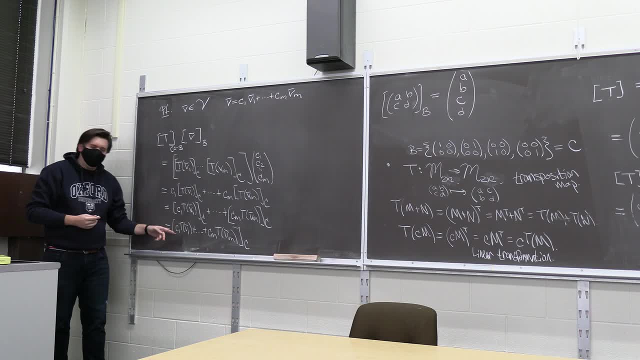 And then what can we say now? What is this guy going to be? the same as Well. T is our linear transformation. So what can you do with linear transformations? You can bring your scalars inside and the linear transformation of a sum. 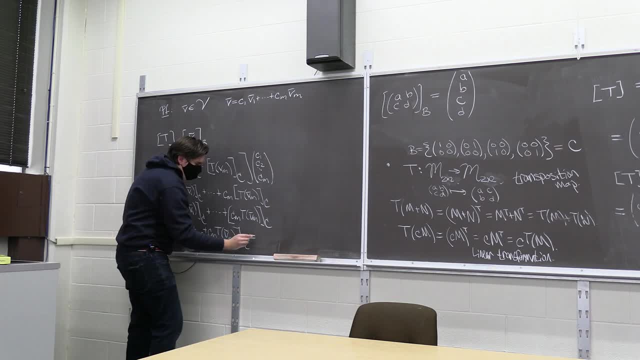 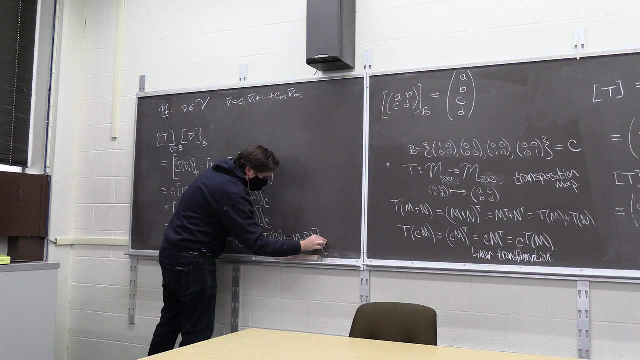 is the sum of the linear transformations. So this becomes just the same as a single T, the transformation applied once to the sum C1, V1 through Cm, Vm. But that's just your vector V. So this is going to give you. 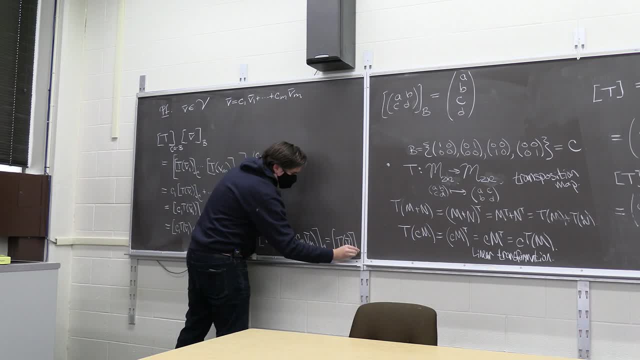 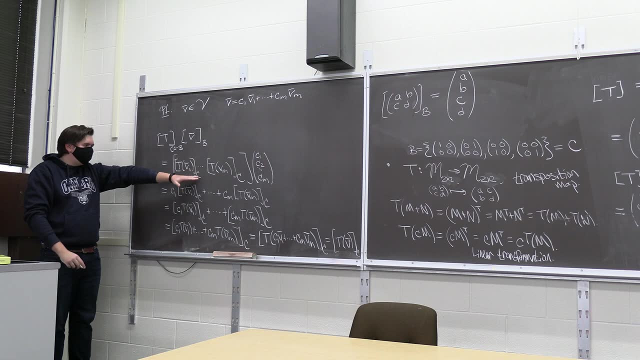 whatever the transformation does to V expressed in your basis C. So, sure enough, this gave us where we wanted to. So this matrix works. How do we know it's unique? Well, this is the same argument that we did before, a very similar argument. 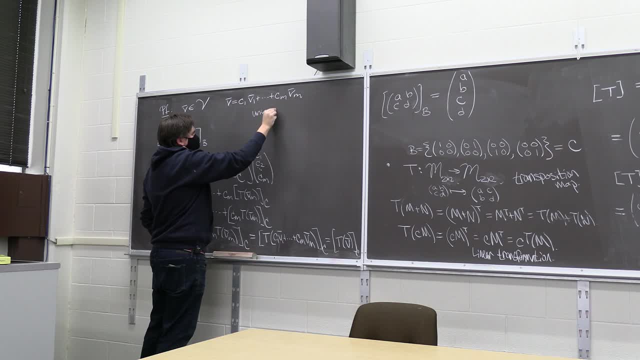 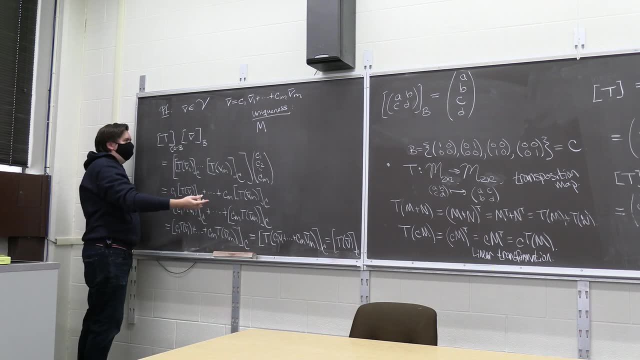 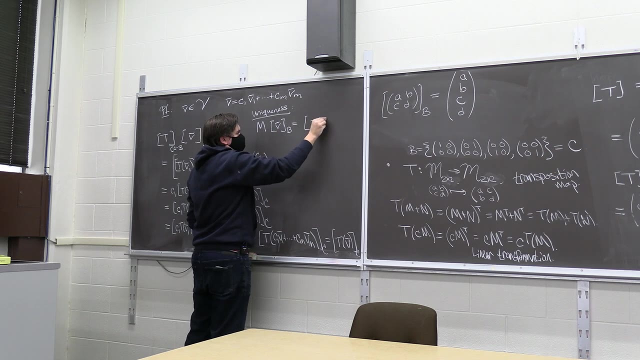 to show uniqueness. You suppose you have some matrix M that does the same thing, so that for any vector V in terms of the basis B, you get out your linear transformation of V in terms of the basis C. Suppose you have a vector M. 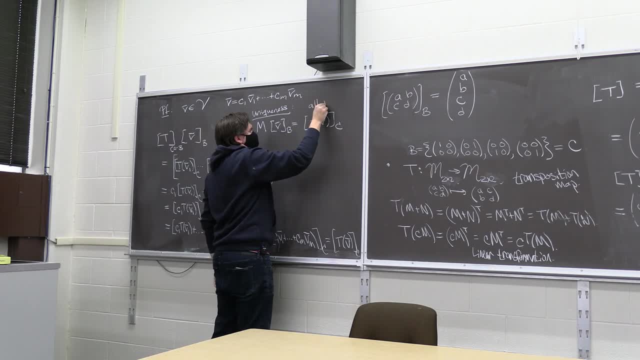 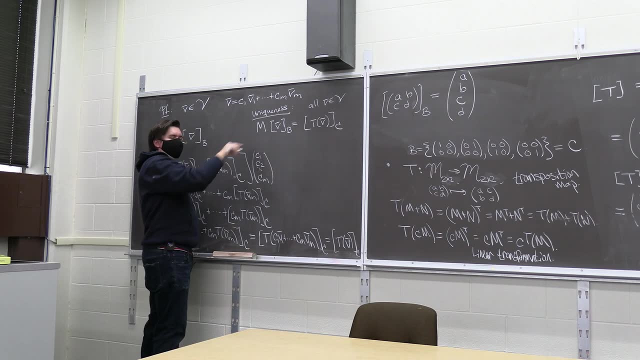 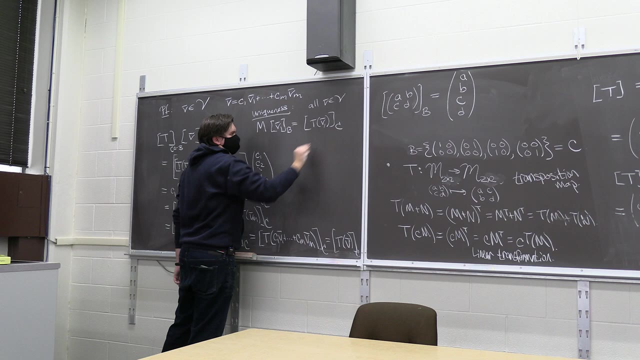 so it's a matrix M that does this for all V in your vector space. And then what do we do? What V in particular should we look at? Yeah, let this be like your V1, the first guy of your basis vector. 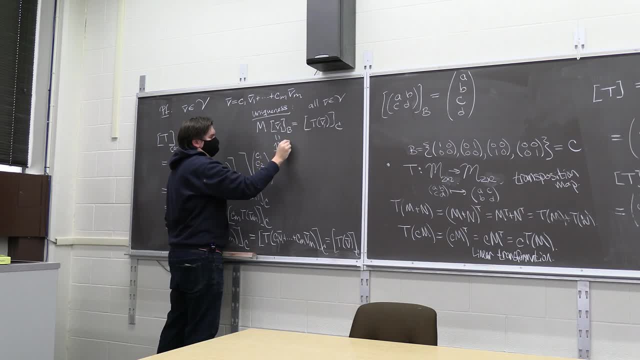 And then remember, this is just going to give you your first column of M, And so you know, your first column just has to be this guy. And in general, if we change this to VI, this becomes the ith column of M, And so you recover it. 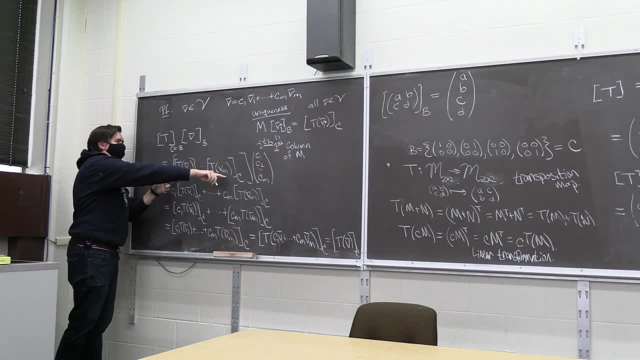 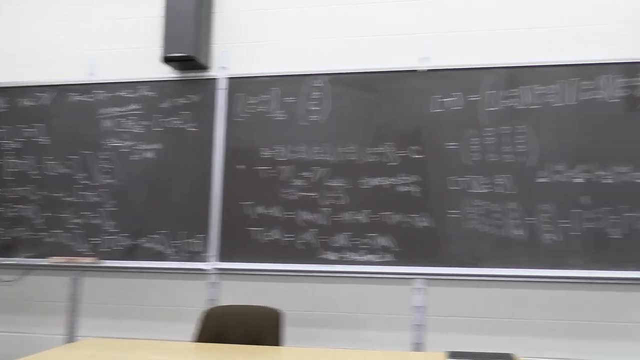 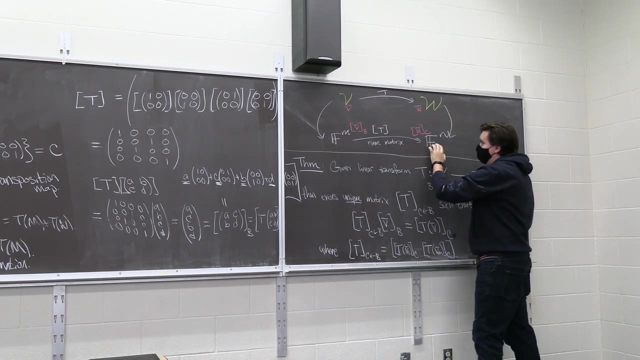 Any matrix that does this has to be that matrix. This is the only matrix. So the big idea is, any linear transformation between vector spaces can be represented by a matrix between these two other vector spaces, which is the coordinates reading off the coordinates of your vectors up here.